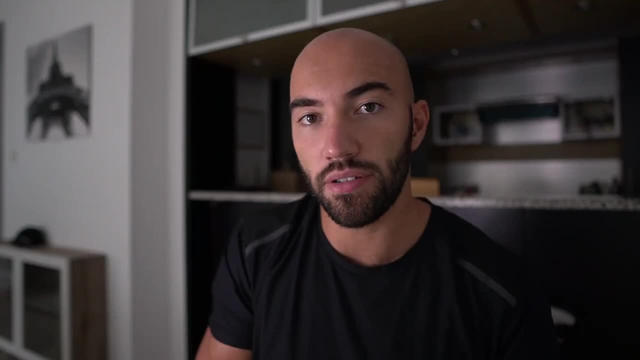 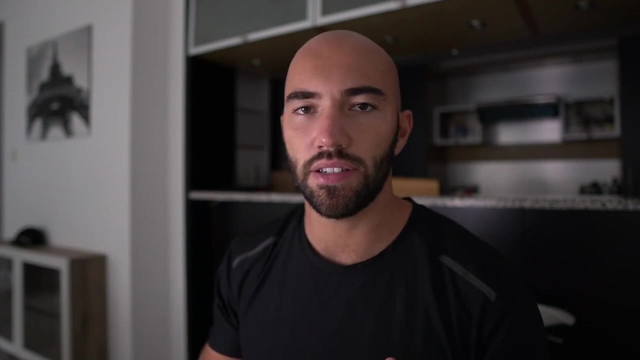 squash them, rotate them, but if a human can still recognize the image, the chances are a well-trained CNN will still be able to identify that image as well. Because of their affinity to image-based applications, we tend to find CNNs being used in image classification, object detection and many other tasks. 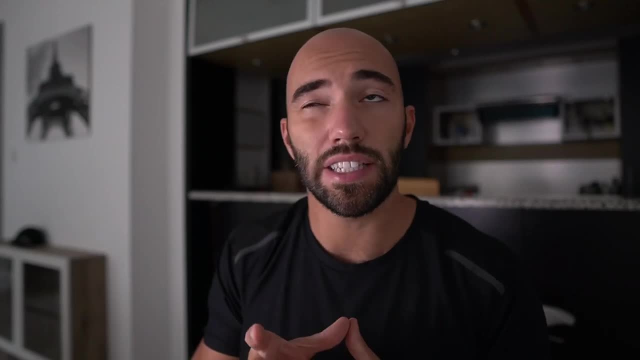 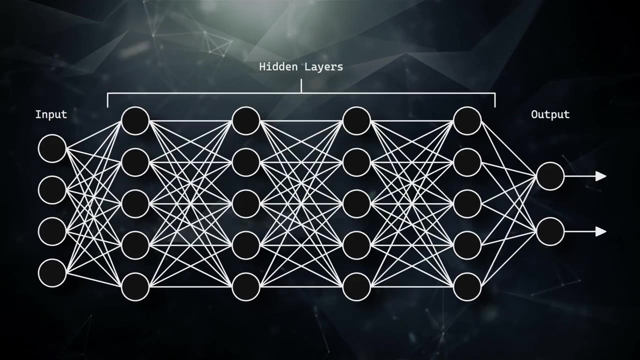 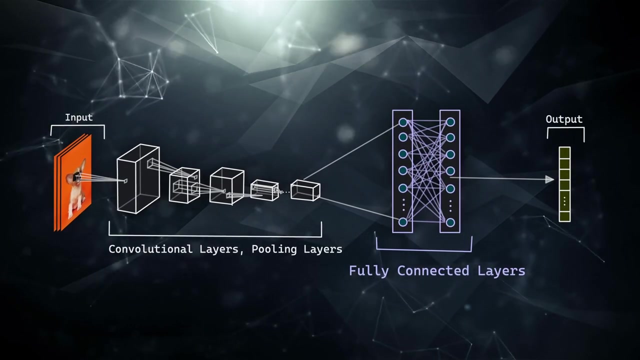 within the realm of computer vision. Now we're focusing on deep-layered CNNs, which are any neural network that satisfies two conditions. The first is that it contains many layers, ie is a deep neural network, and two, that it contains convolutional layers. Beyond that, convolutional neural networks can. 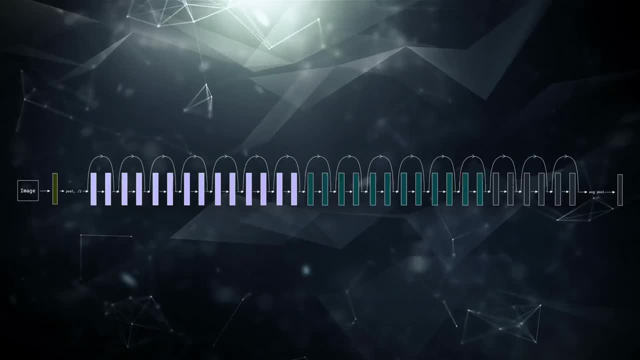 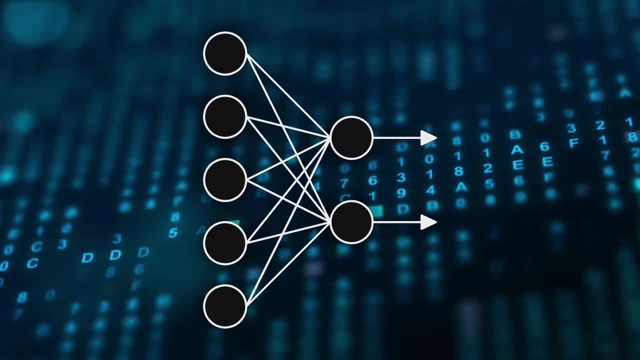 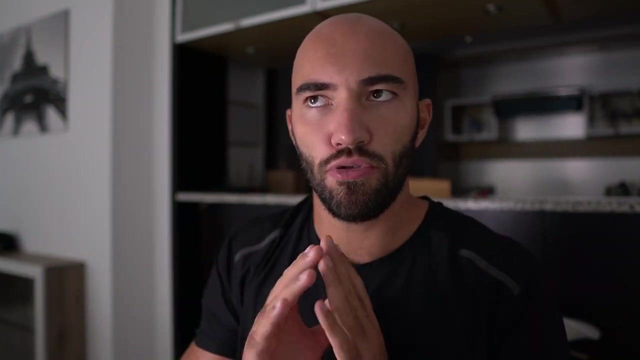 consist of many different architectures and they will contain many different features. Common ones include pooling, normalization layers and also linear layers, And we'll see a few examples of the different types of convolutional neural networks later on in a video. Now let's just briefly focus. 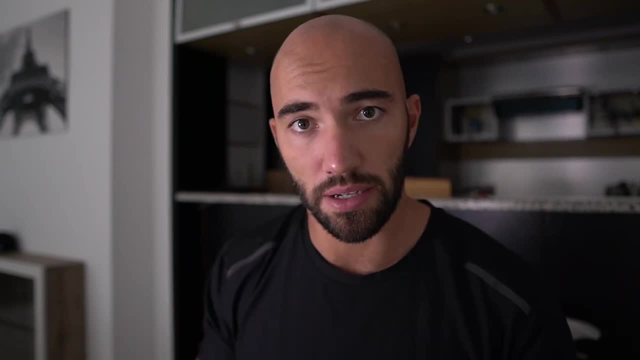 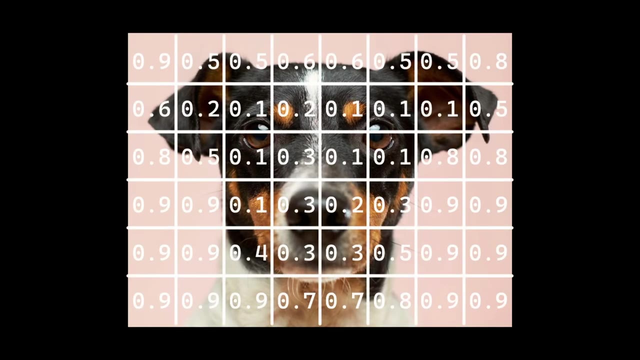 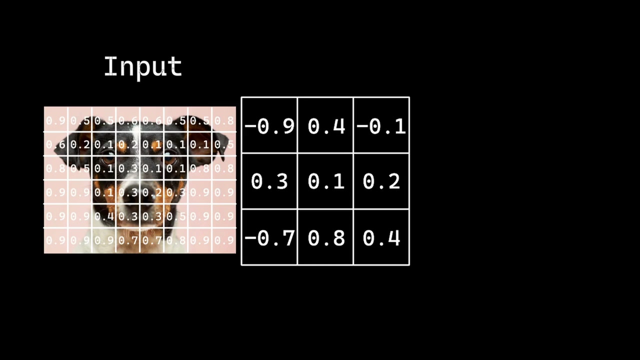 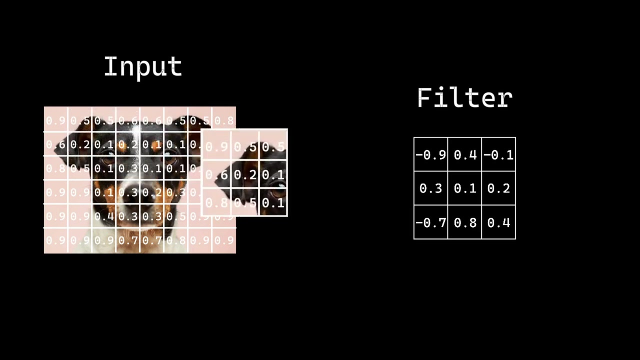 on what exactly a convolutional layer is actually doing. So we can think of an image as a big array of activation values. These arrays are followed by many more arrays of initially randomly initialized values, The weights that we call a filter or a kernel. A convolutional layer is nothing more than a. 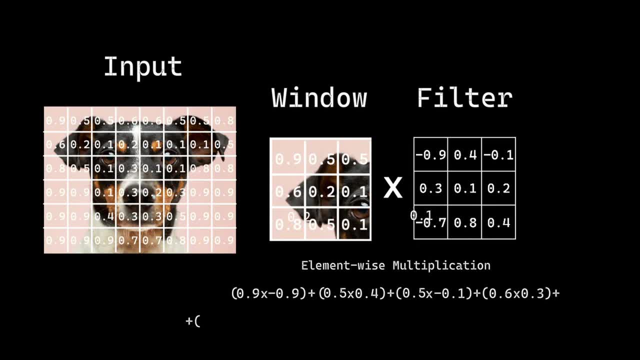 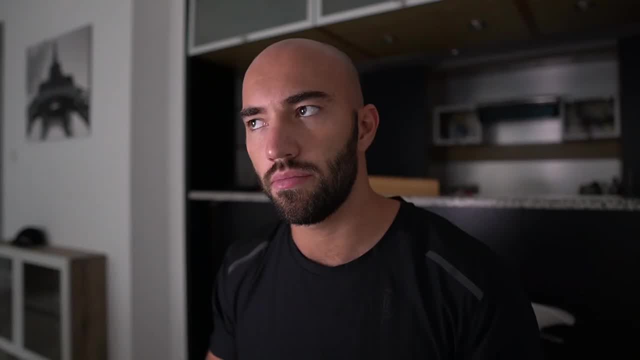 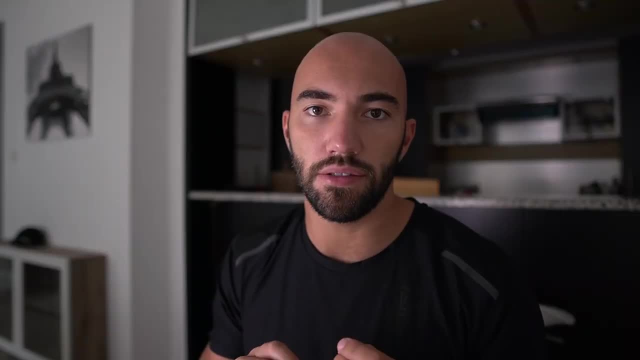 element-wise multiplication between these pixel values and the filter weights, which are then summed together. This element-wise operation, followed by the sum of the resulting values, is often called the scalar product, because it results in a single scalar value, And we can see how that works here. So we have 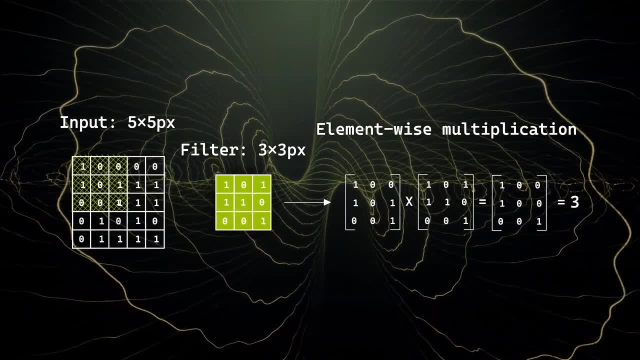 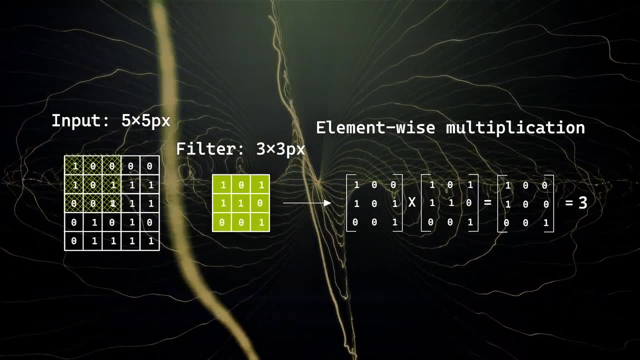 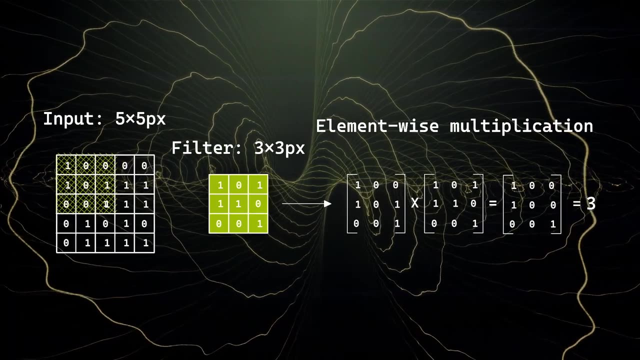 our input, which is a 5 by 5 pixel image, and we have our filter, which is 3 by 3 pixel. Correct, In this very first iteration of the convolution, we can see that we are multiplying the 3 by 3 window within that input by the filter weights. 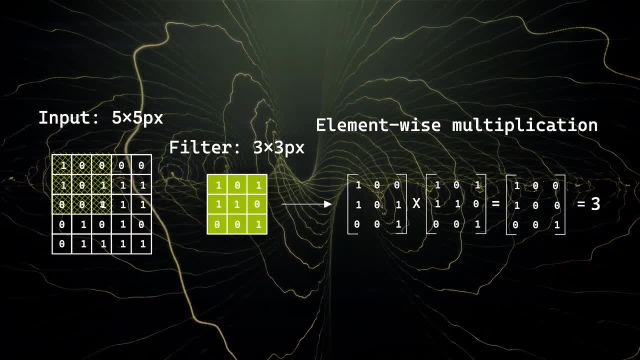 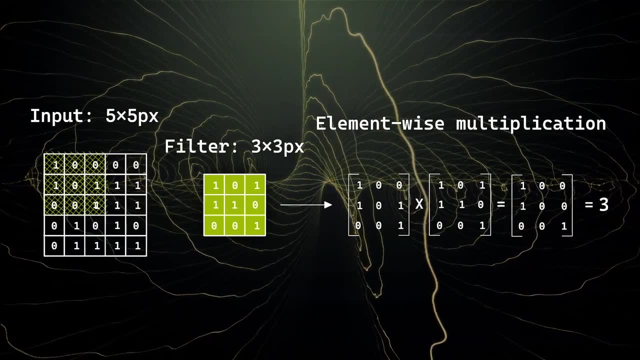 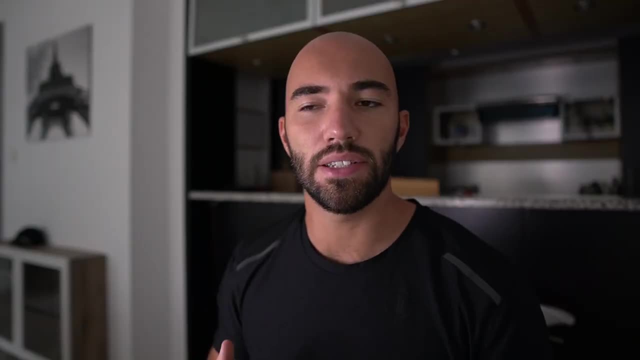 Multiply both those together in element-wise multiplication to get the array that you can see on the right In there. we can see that the sum of all values within that array is equal to 3, and that is our scalar product value. Now, in reality we would not. 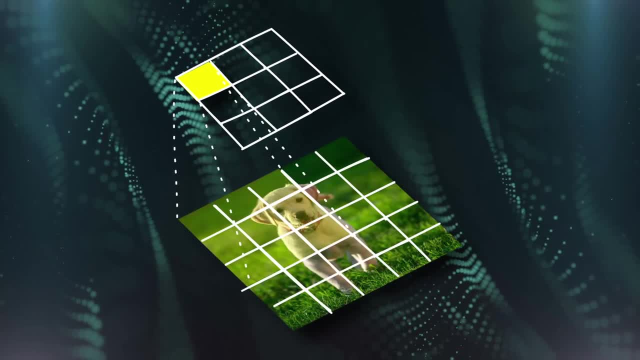 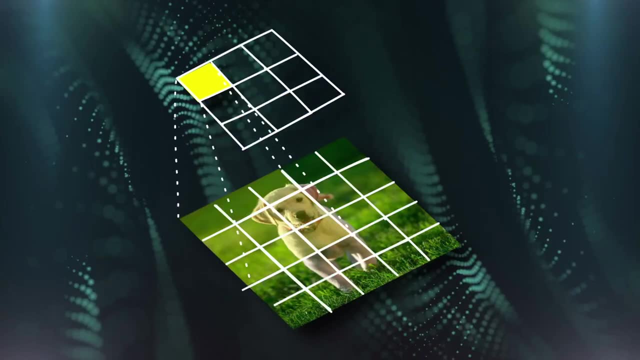 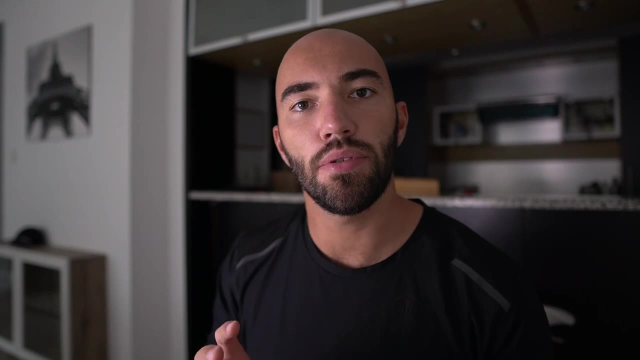 just return a single value, because we would actually be sliding this window, this filter, over the full image And the output of each one of those window operations is a single value. but of course we now have nine values from this larger image. Now the output of this convolution is what we would call a. 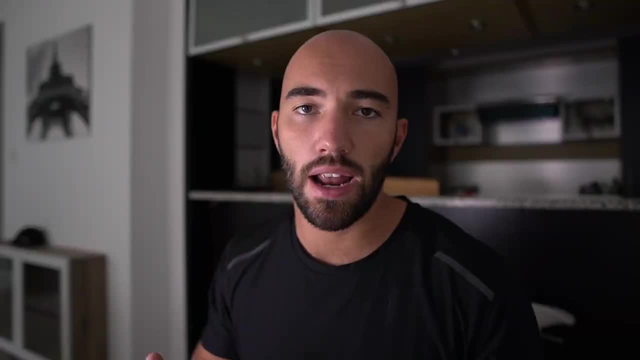 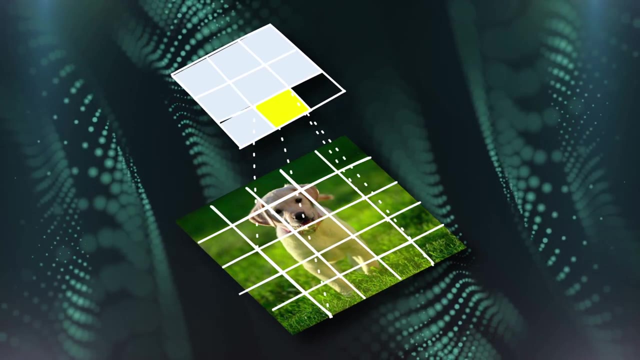 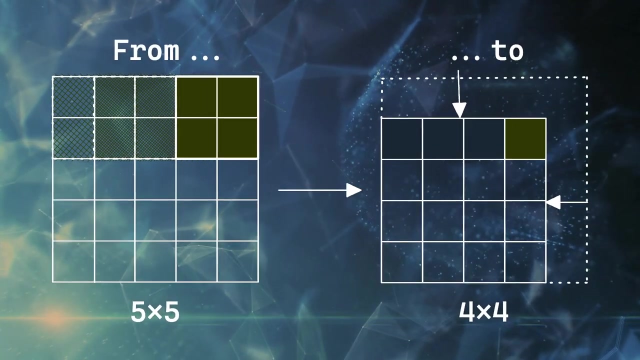 feature map or an activation map. Both mean the same thing And we call it like that because it is a mapping from the activations of detected features, from a filter to the input layer. Now, something worth noting here is, obviously we are going from a larger dimensional space into a smaller dimensional space. We're 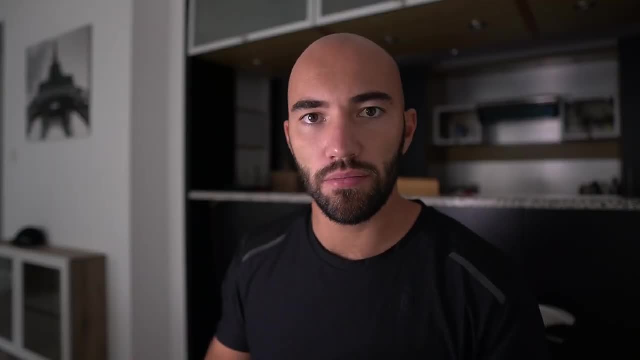 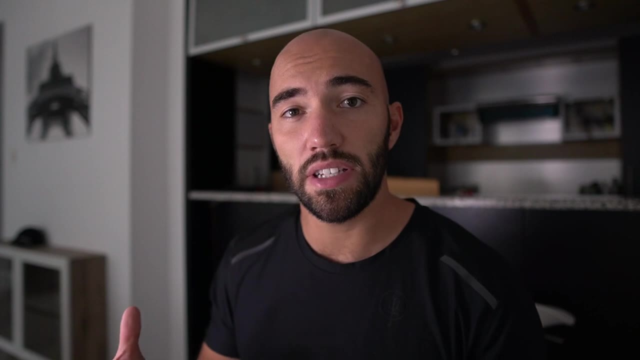 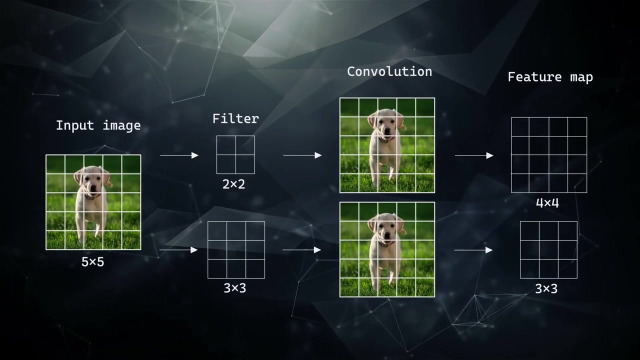 compressing that information. So we always need to be mindful of excessive compression and therefore data loss via dimensionality reduction, And because of this we may want to increase or decrease the amount of compression that our filters create. To do that, we modify the filter size and also how quickly. 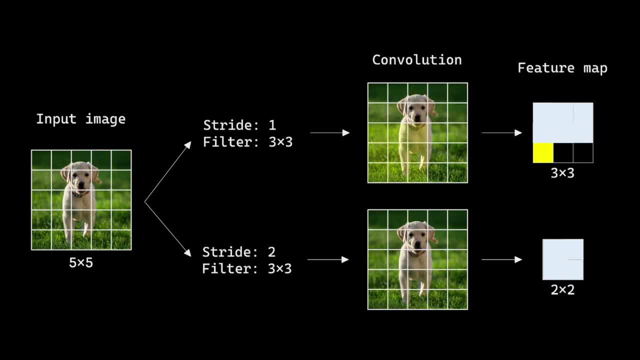 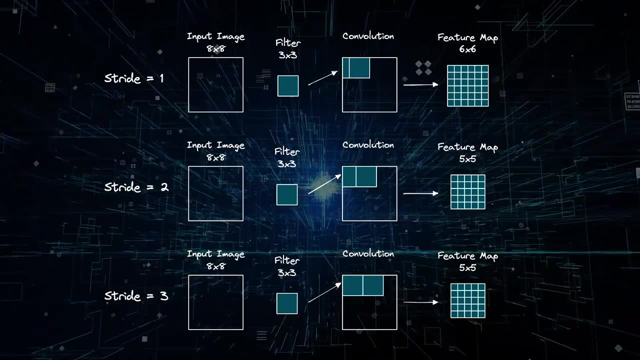 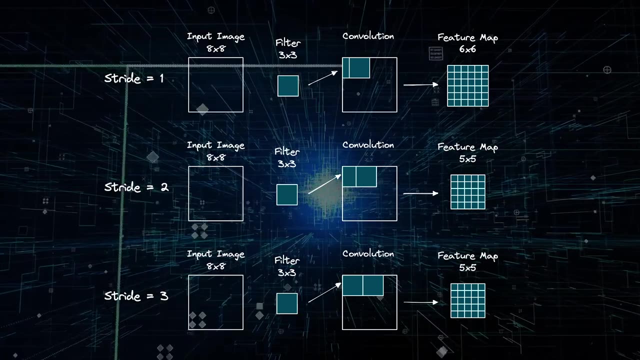 it moves across the image using a variable called the stride. The stride defines the number of pixels a filter moves after every calculation. By increasing the stride, the filter will move across the entire image in fewer steps, outputting fewer values and producing a more compressed feature map. 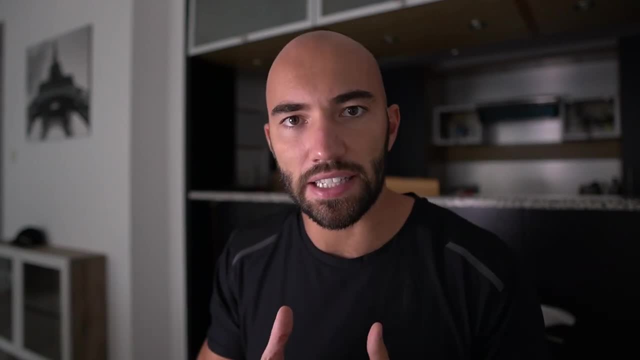 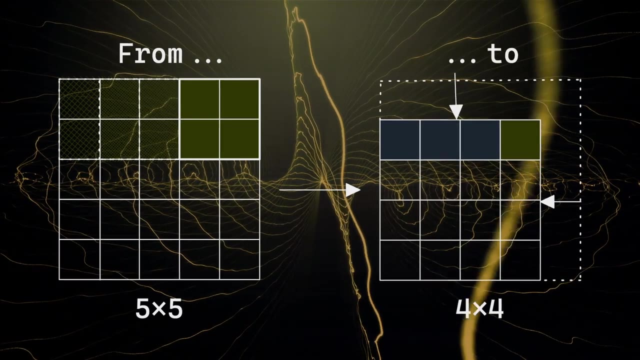 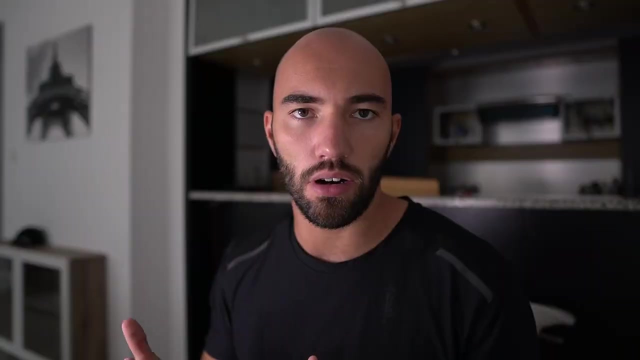 Now there are also some other surprising effects of image compression that we need to be aware of. One of those is the filters interaction with the border areas of a input image or input array. If we're not careful with this, the border effects on small images can result in a rapid loss of information. 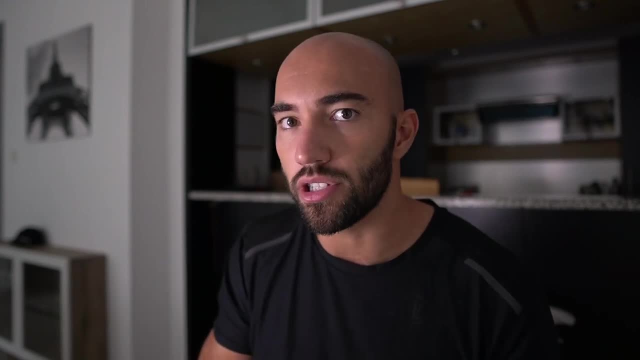 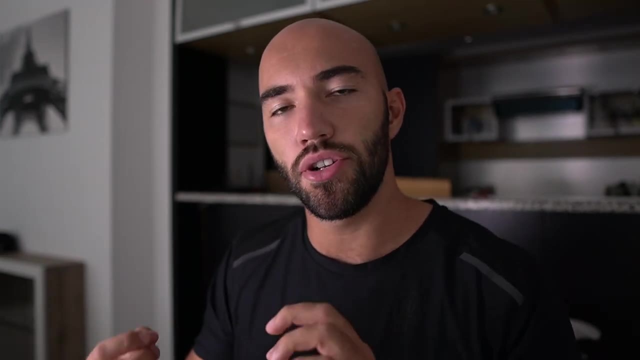 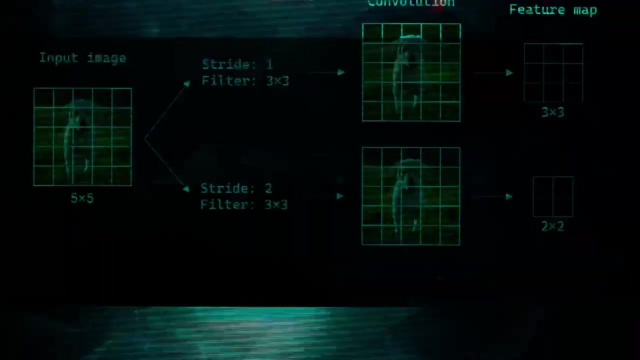 And that's naturally more of a problem for those smaller images, because they start with less information in the first place. So to avoid this, we must either reduce the amount of compression that we're doing using the previous techniques that we mentioned, So being mindful of the filter size and the 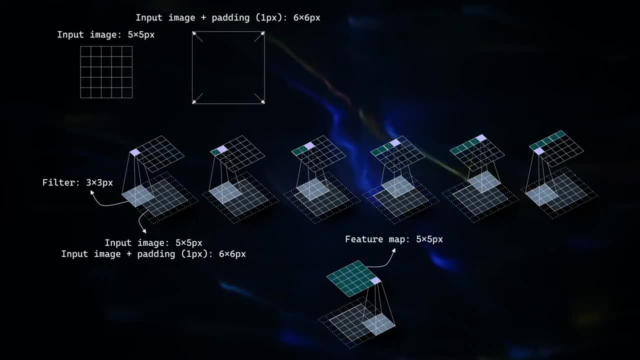 stride, or we can add padding. Now we can see the effect of padding here. so we are essentially taking the original image and we're adding padding around the edge of the image. Now, typically this padding is going to be a set of zero value pixels and we add that around the image to limit or prevent compression between. 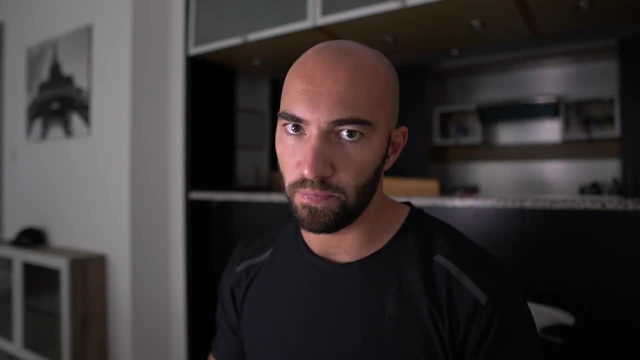 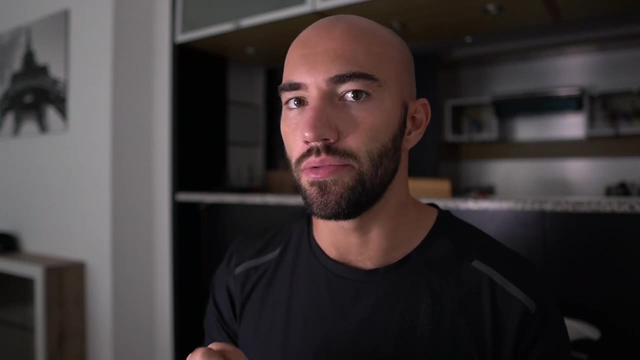 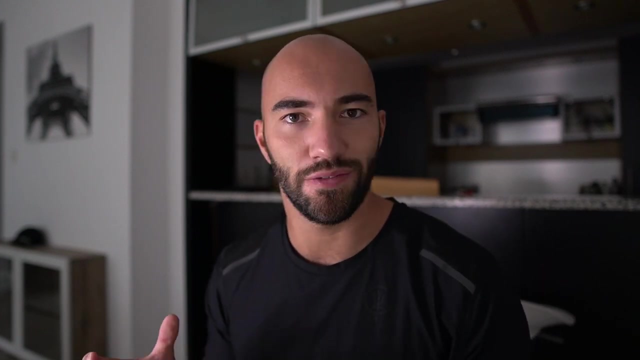 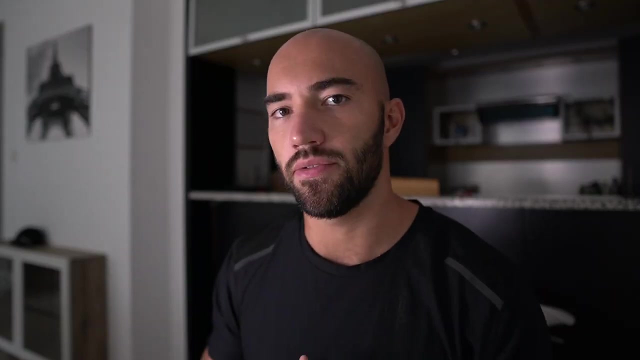 layers. For larger images this is going to be less of a problem, but for those smaller images, padding is very effective remedy to avoid too much information loss. Now, another key feature of these deep convolution neural networks is obviously depth of those networks. Going way back to 2012, the first very successful convolutional neural network, 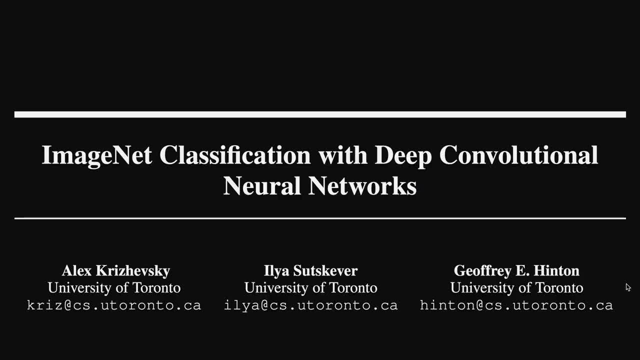 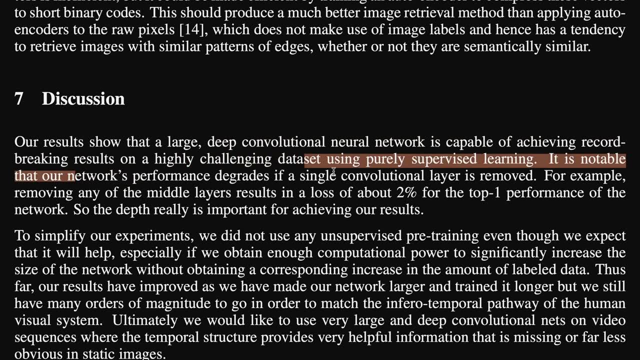 or deep convolutional neural network, was called AlexNet, and the authors of AlexNet found that the depth of their network was a very key component that contributed to its high performance. The reason for this is every successive layer within a convolutional neural network abstracts the initial. 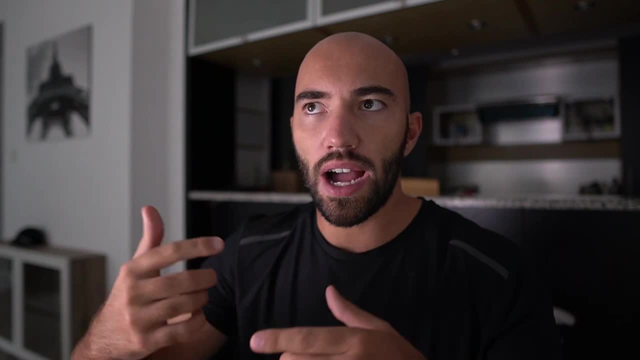 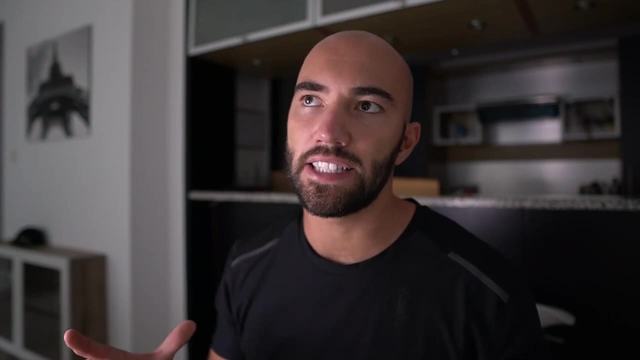 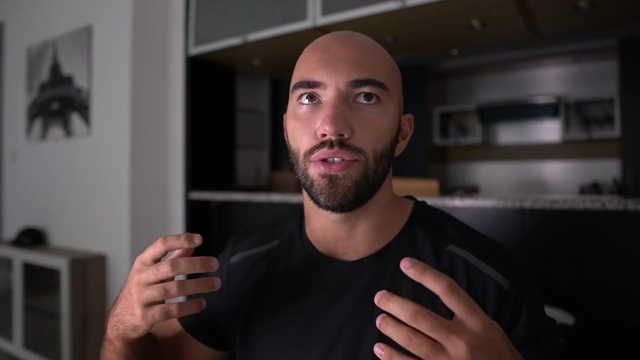 features more and more, so we get more and more abstract features as the number of layers within the network increases. We can think of this as the network is able to abstract image features more and get them closer to the very abstract layers of a dark fields basically. So this often results in misapplication of 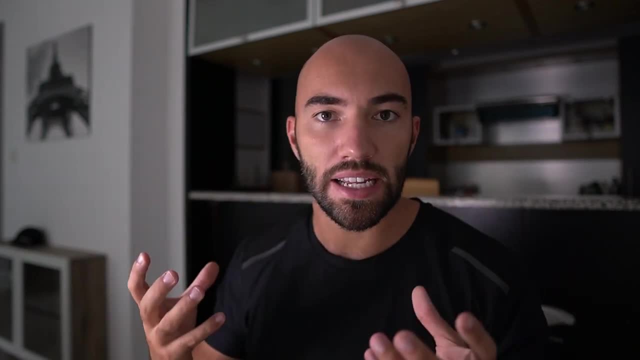 cast colour in aarpぁ. result, which may not be ait from the bottom, but rather causes presentation Chair and the in the average reality, that the size of these abstract concepts that we have in our minds as human beings, so it gets closer to a human-like. 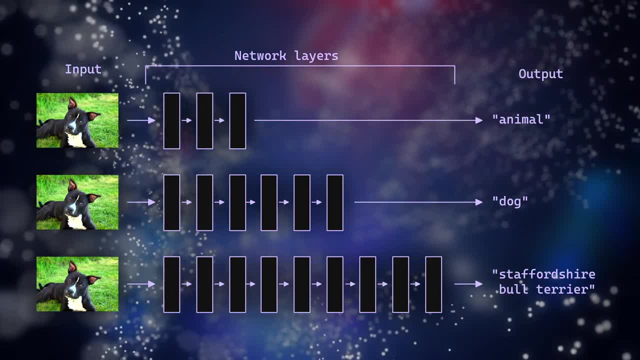 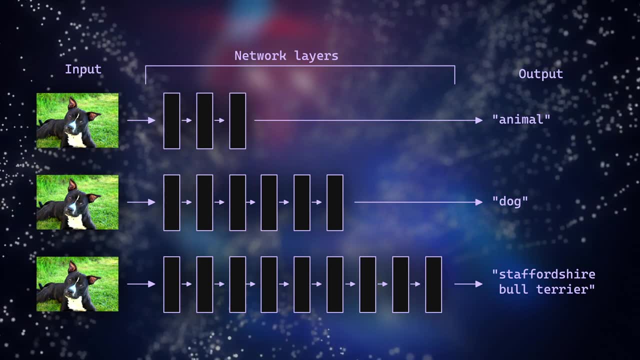 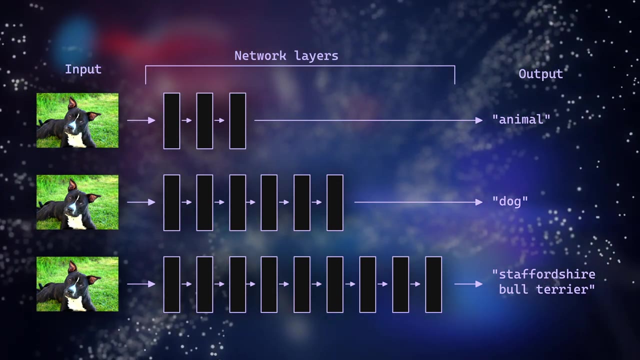 understanding of an image. So, for example, a shallow CNN might recognize that an image contains an animal, but as we add another layer it may be able to identify that animal as a dog. It has become more abstract and adding another layer may allow that network to identify specific breeds, like a. 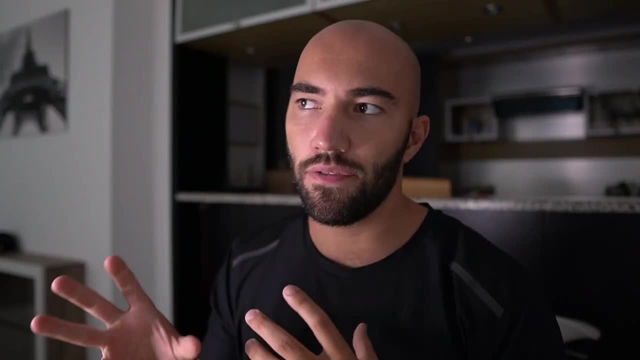 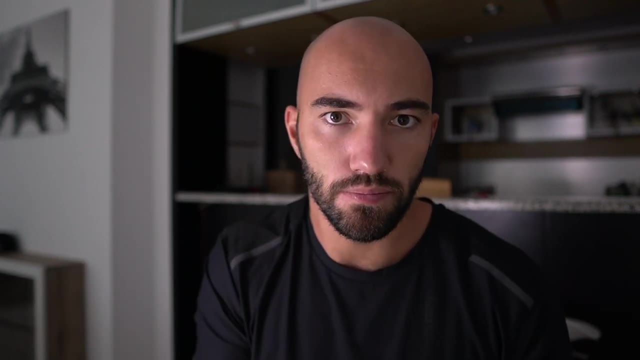 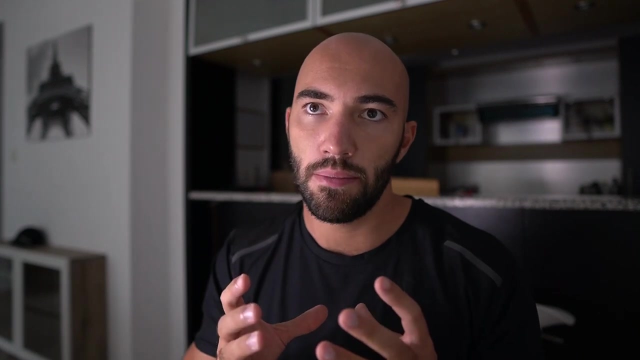 bull, terrier or a husky- These ideas of different dog breeds- is far more abstract than a dog or just an animal and it requires far more abstraction in order to actually understand that and for CNN to be able to identify that. So by adding more layers, we're generally going to be able to identify. 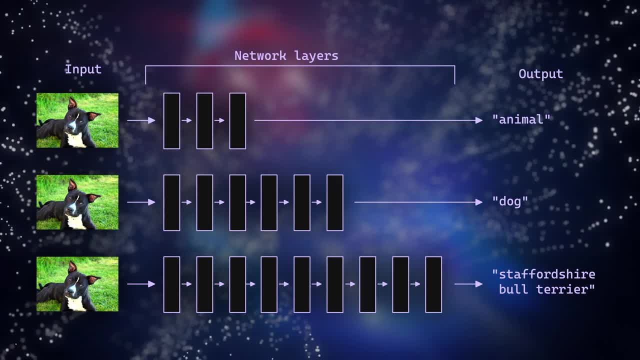 more abstract and more specific concepts Now moving on to what are the most important concepts in our minds. So we're going to be able to identify more abstract concepts Now moving on to what are the most important concepts in our minds. So we're going to 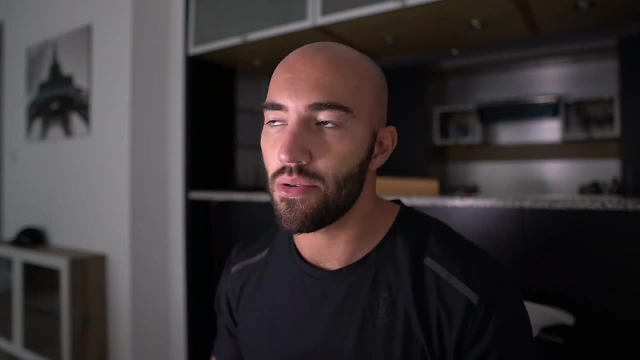 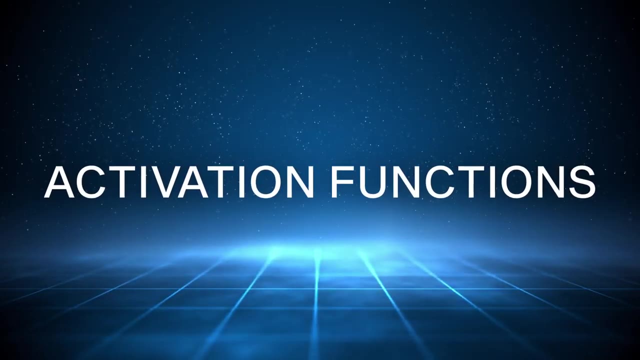 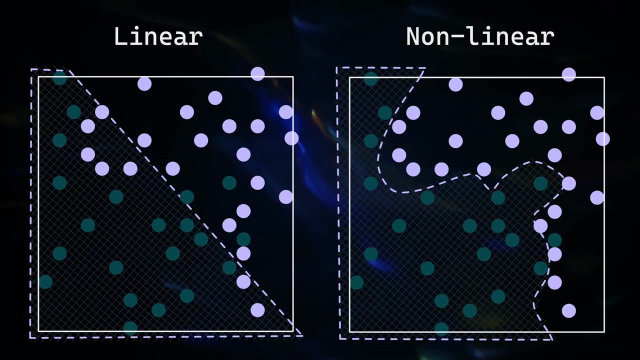 are some of the very common features of a convolutional neural network, although not necessarily restricted to convolutional neural networks alone. We have activation functions. So activation functions- we will find that in pretty much every neural network and they are used to add non-linearity to these networks and essentially what that allows us to do, particularly over many 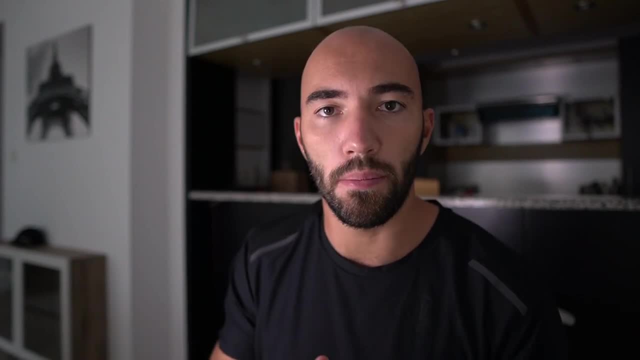 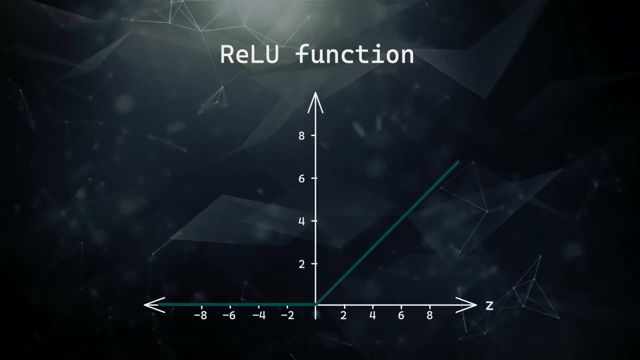 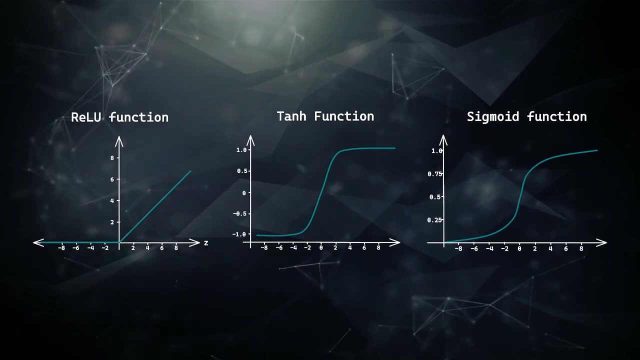 layers is represent more complex patterns. Now you may recognize a few of these things, but these activation functions. we have the rectified linear unit function, the tanh function and sigmoid function. These three are some of the most common activation functions that we find in neural networks. 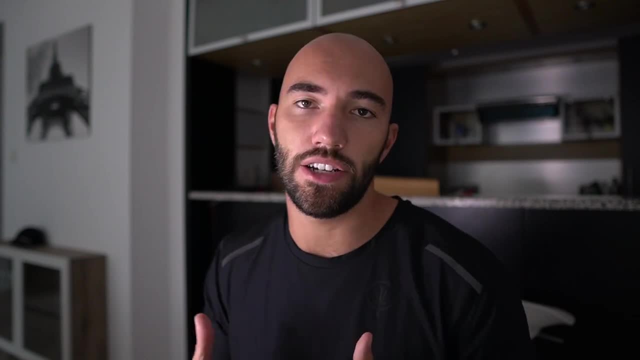 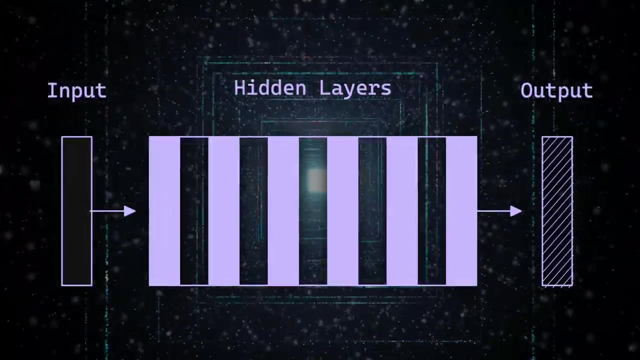 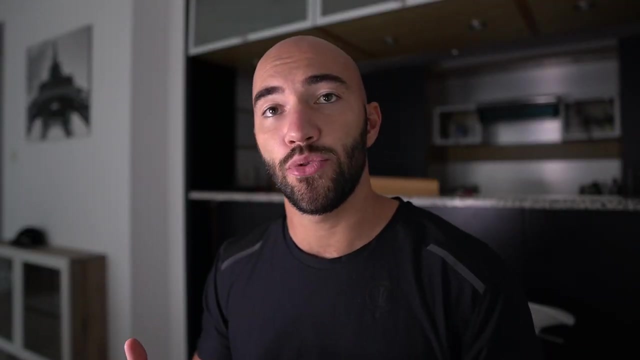 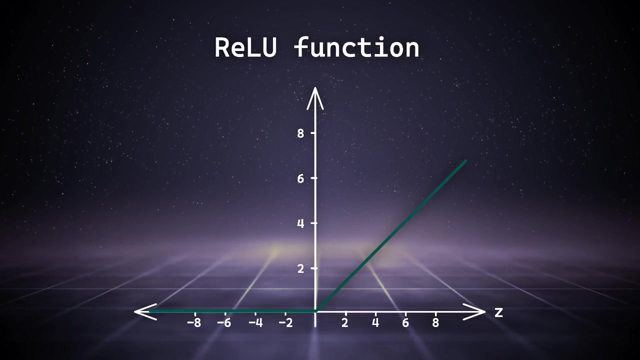 In the past, CNNs often use activation functions within the hidden layers of the network, so that the middle layers of that network- basically not the input or the output, everything in between- and they will typically use tanh or sigmoid activations. However, in 2012, the rectified linear unit activation function became very popular because it was used. 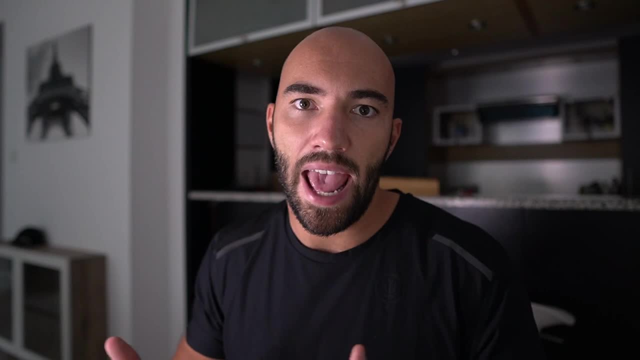 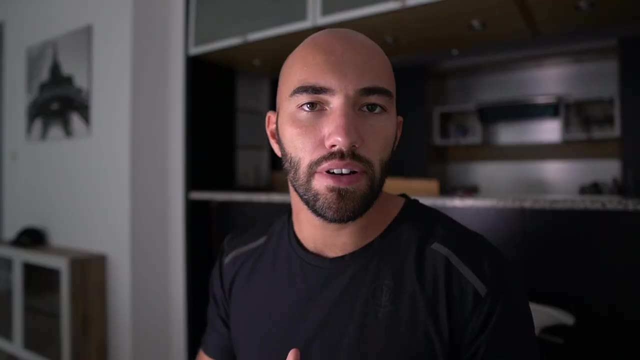 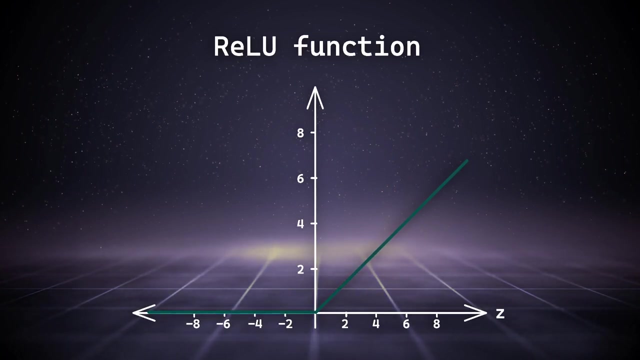 by the AlexNet model, which kind of kick-started this era of deep learning, as it was the best performing CNN of its time by a longshot. Nowadays, the rectified linear unit, or rally unit, activation function is still a very popular choice. It's a lot simpler than tanh and sigmoid and 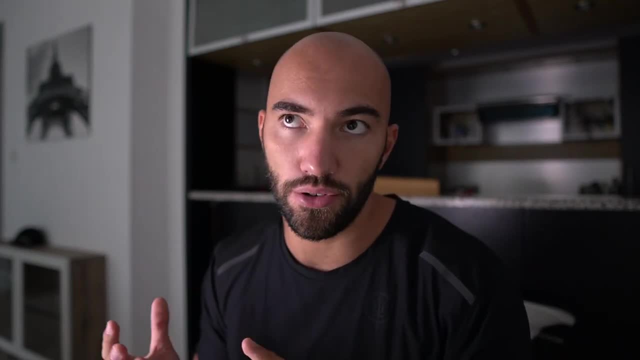 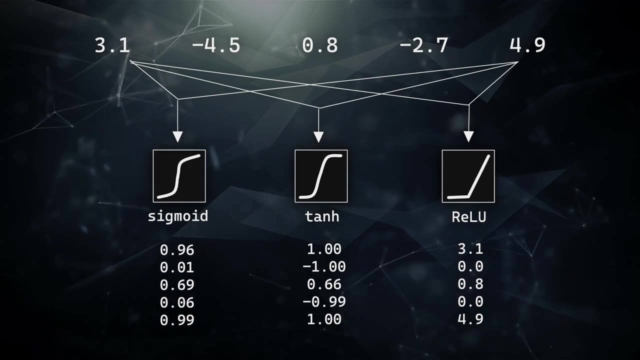 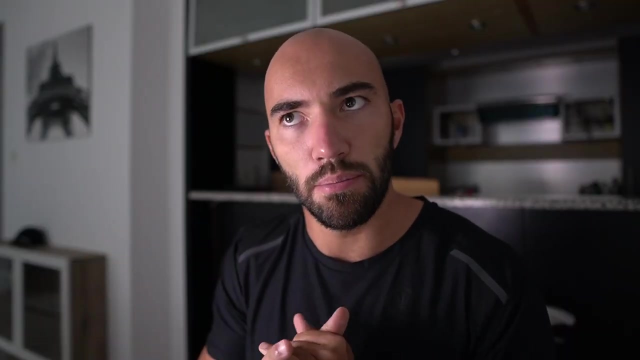 also doesn't require any case reporting of a дальше such an activity. The only thing I require regularization in order to avoid saturation, which basically means the congregation of activation outputs towards the minimum maximum values of that activation function. Another very important feature is the use of pooling layers. Now, we use pooling layers because the output of 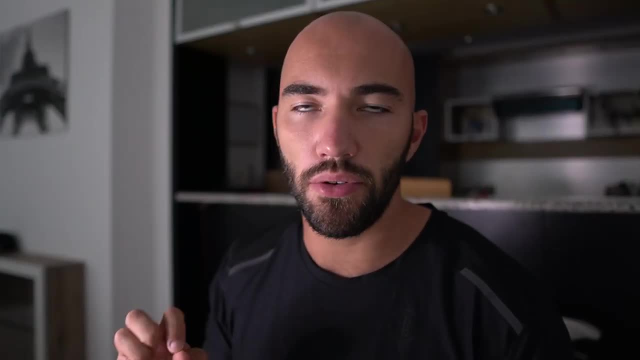 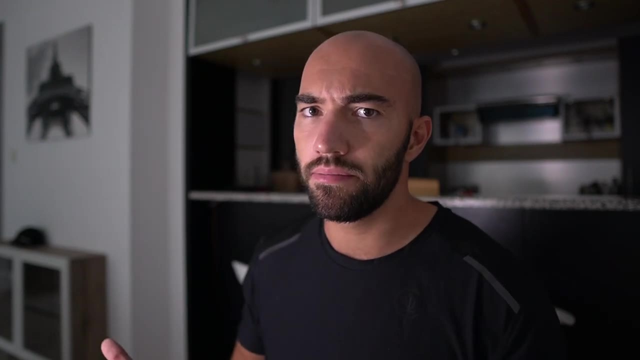 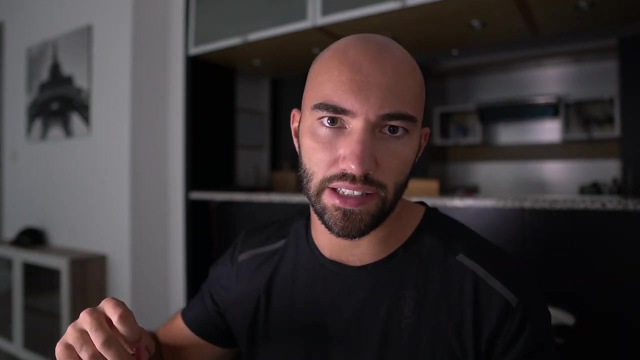 feature maps are very sensitive to the location of input features, so a small change can make a big difference. To some degree, this can be useful, as it can tell us the difference between, for example, a cat's face and a dog's face, based on where the eyes are, where the ears are, and so on. 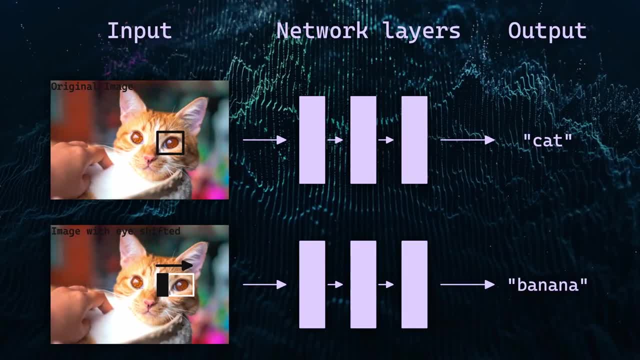 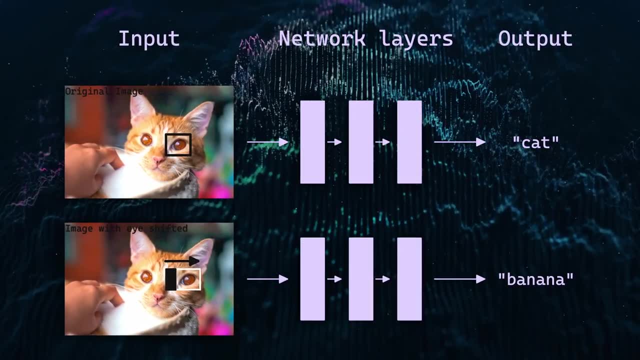 However, we don't want that to be too dramatic because if an eye is shifted two pixels to the left or two pixels to the right, that should still allow the model to identify this image as being of a face. It should not make it go crazy and detect something completely different. and we 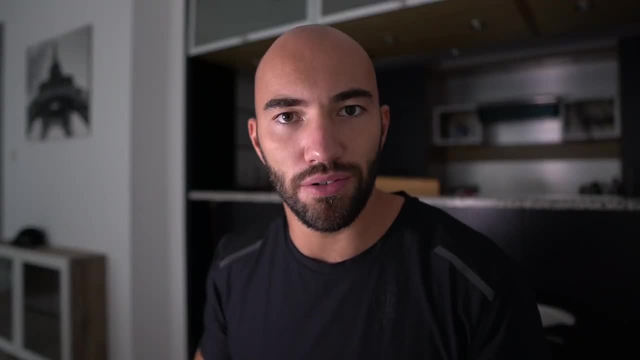 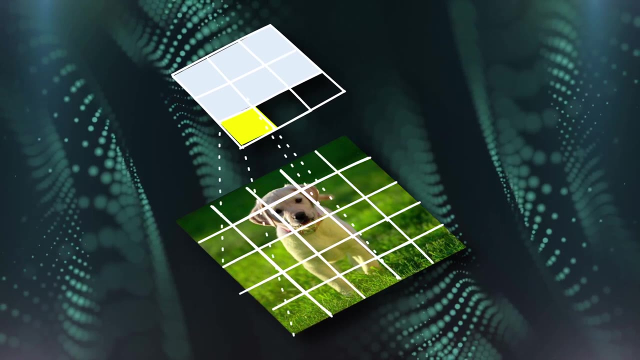 need to be able to identify this image as being of a face, So we need to be able to identify this pooling layers in order to allow the model to have this form of smoothing or stability. Pooling layers are a downsampling method that compress information from one layer into a smaller space. 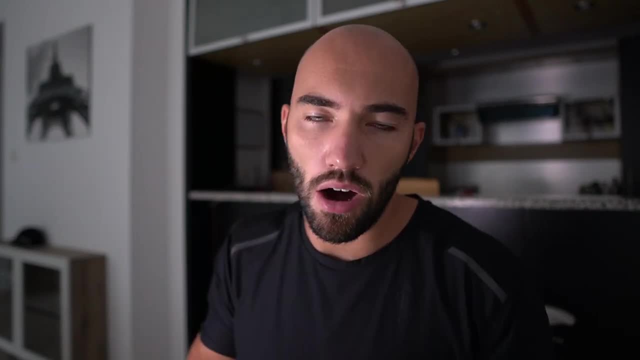 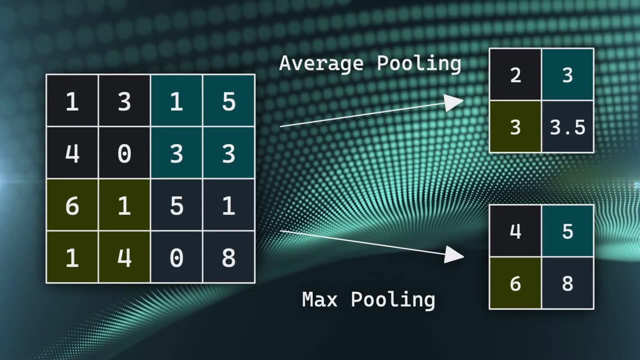 in the next layer, and the two most common pooling methods are max pooling and average pooling. Max pooling takes a maximum value of all the values within a window and average pooling takes the average of all those values. So the average pooling takes the average of all the values within a. 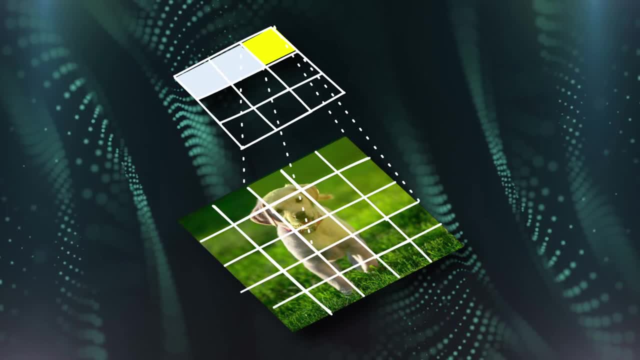 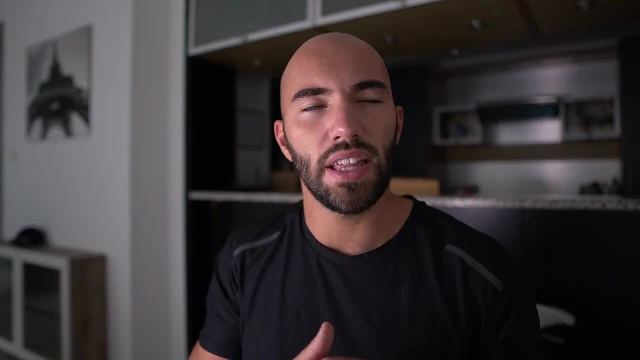 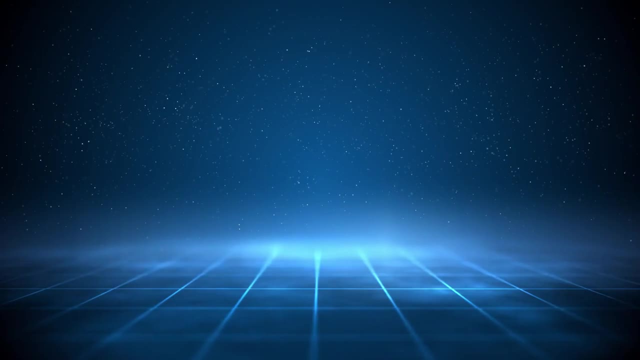 window And, of course, as that pooling window moves across our input array, we would end up outputting another array of smaller dimensionality, And with that we can move on to the final main feature of a convolutional neural network, which is the use of fully connected layers, A fully 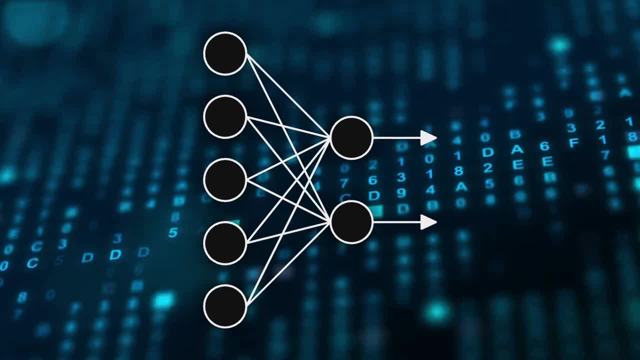 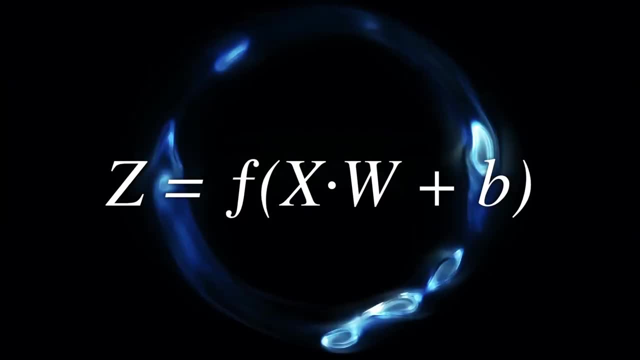 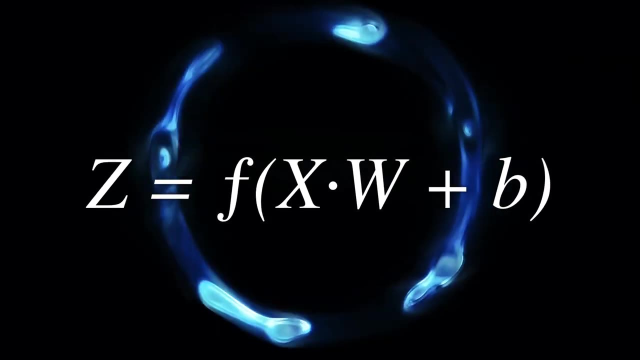 connected linear layer is simply a neural network in the very traditional stripped down sense. It is the dot product between some inputs and some outputs And the dot product between some inputs, X, and the layer weights W, with a bias term added onto there and usually an activation function. We 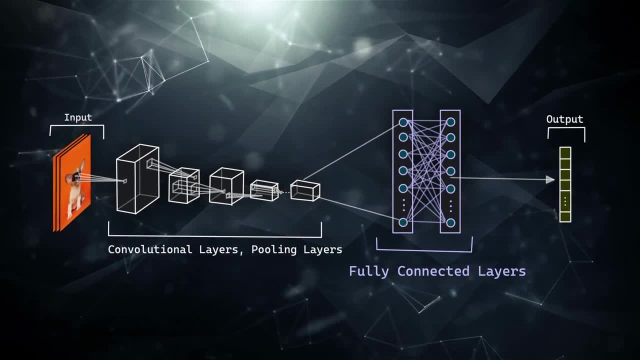 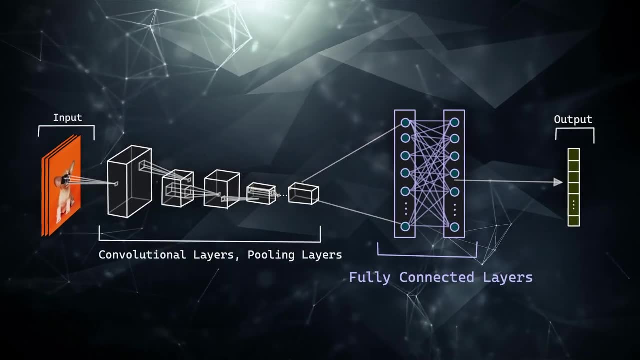 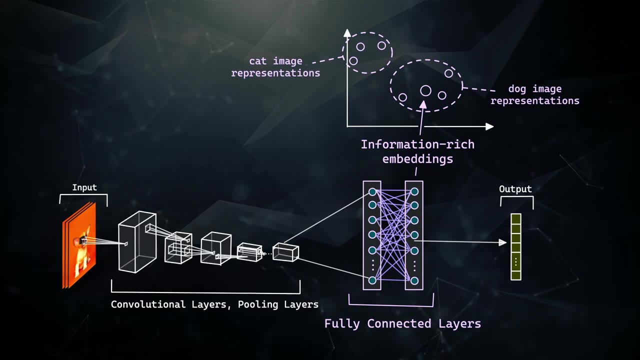 will typically see a fully connected layer at the end of a convolutional neural network and it handles the transformation of our convolutional neural network embeddings from 3D tensors to more understandable outputs like class predictions. It is often within these final layers that we will 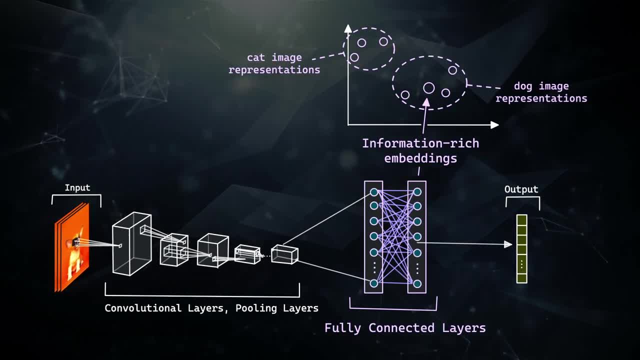 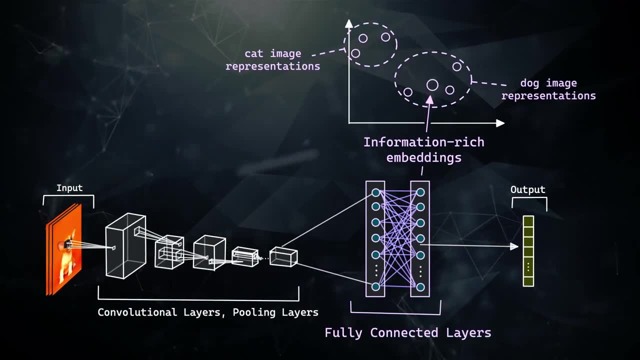 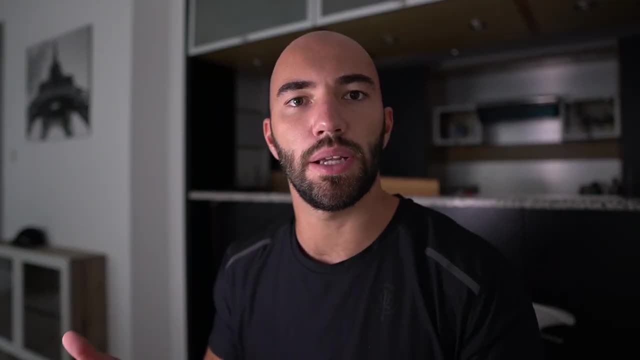 find the most information rich and reliable. The most important thing about convolutional neural networks is that they have rich vector embeddings that represent the information that has come through all of those layers and have the most abstract, machine readable numeric representation of whatever image is being passed through all of those layers, And it's this that we will typically 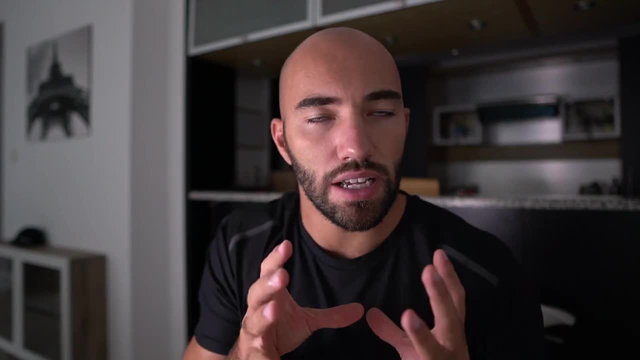 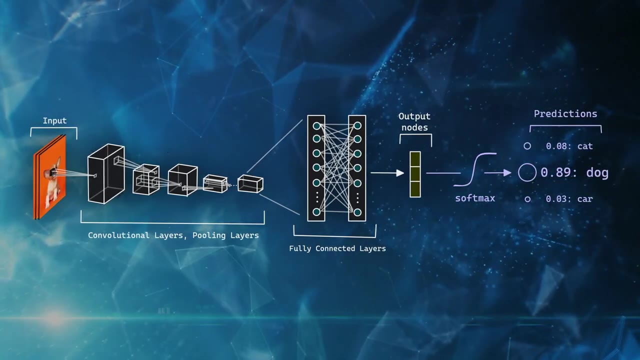 use in things like image retrieval. But focusing on the classification, what a classifier will usually do is apply a softmax activation function and that will create a probability distribution across all of the output layers within the convolutional neural network. And that will create a probability distribution across all of the output layers within the convolutional neural network And that will 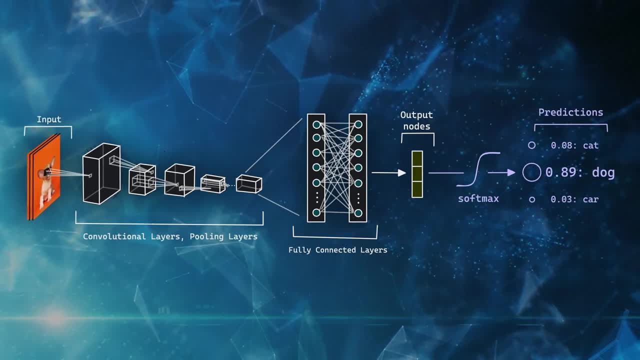 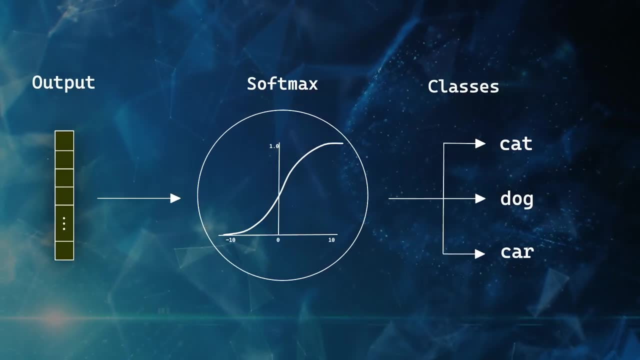 create a probability distribution across all of the output layers within the convolutional neural nodes, where each one of these nodes represents a candidate class or a potential label. For example, here we have cat, dog and car. Those would be our output classes And after these fully connected. 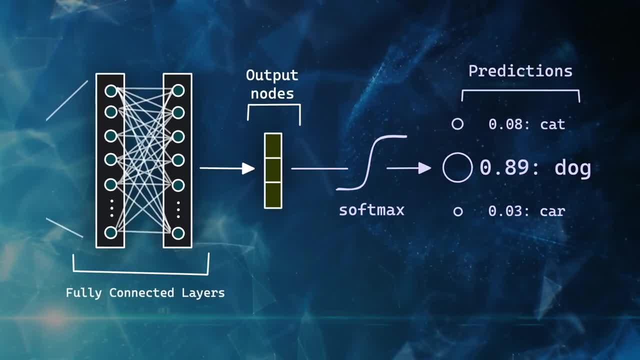 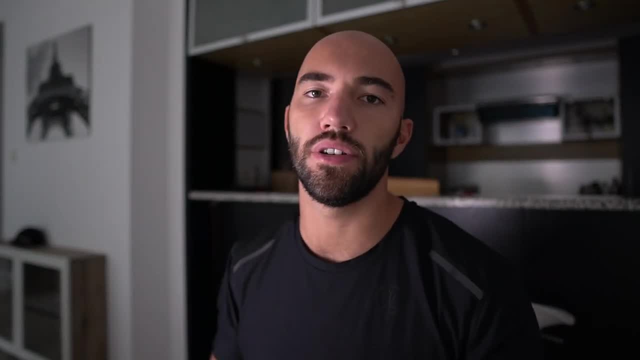 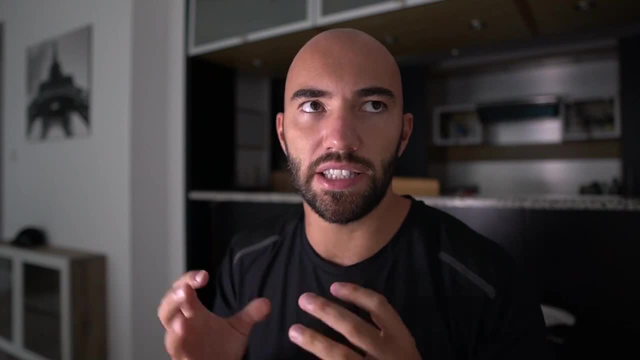 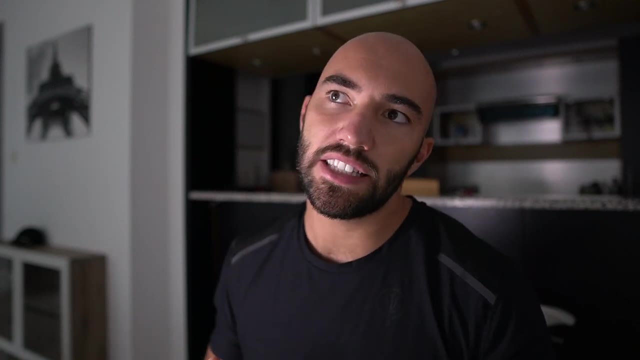 many different convolutional networks have been designed, So there is no specific architecture, but instead what we can use is some of the most high performing networks as almost a set of guideposts in how we can design our own networks or simply use those existing networks. 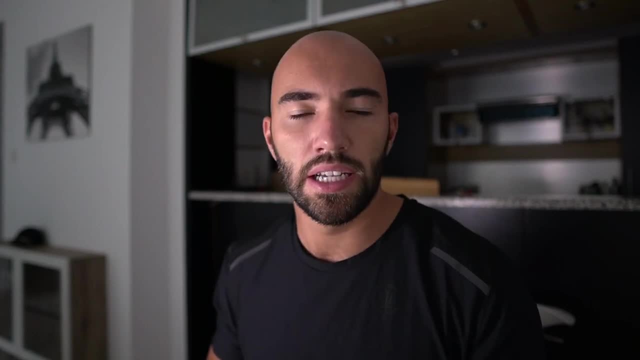 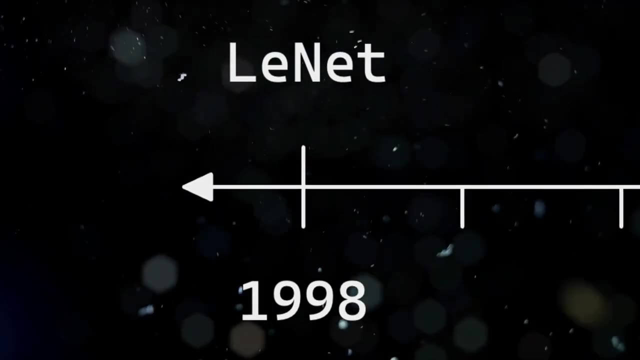 So to have a very quick high level, look at a few of the most popular ones. So we'll start way back when, with the very first successful convolutional neural network, which was LeNet. Now LeNet is a very popular neural network And is one of the most popular neural networks in the 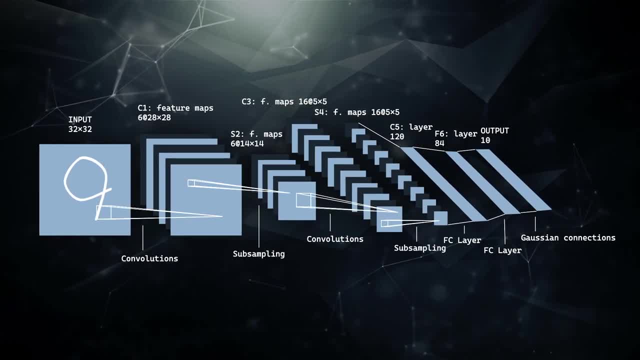 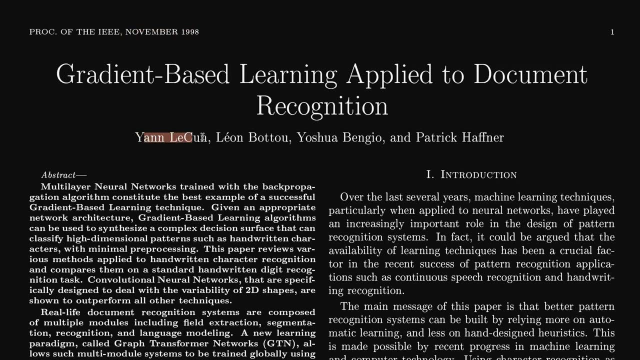 LeanNet is, I think, the earliest good example of a deep convolutional neural network being applied in the real world. It was developed in 1998.. And in reality a lot of us have probably actually interacted with LeanNet without ever even realizing. 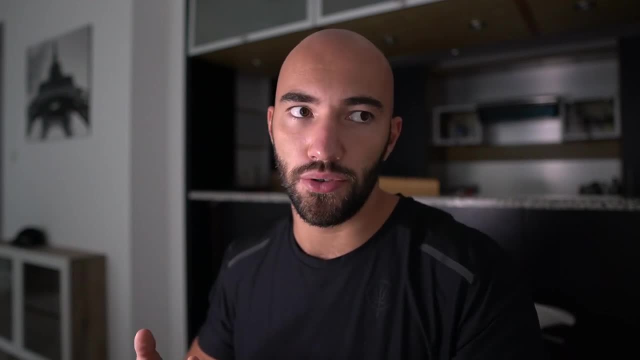 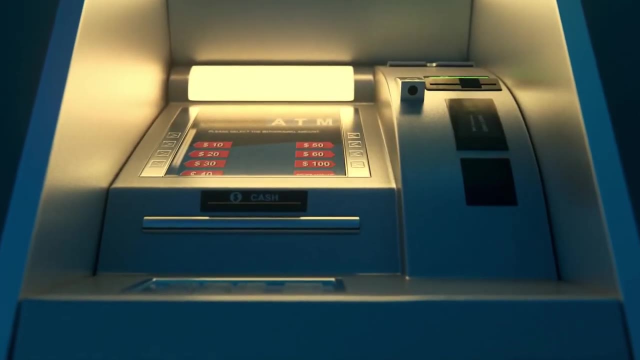 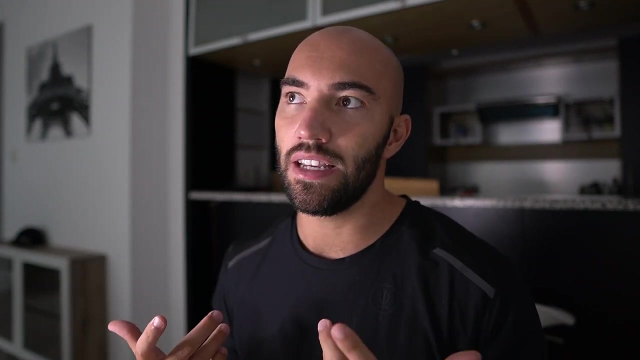 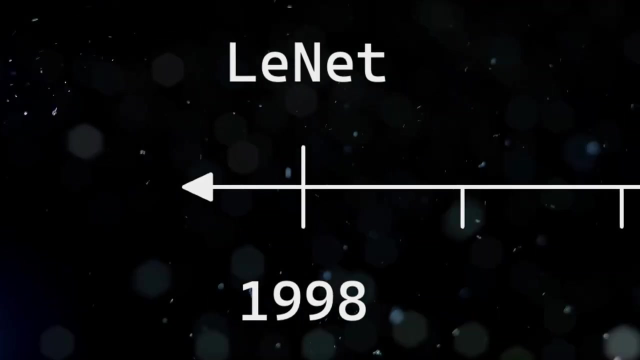 It was developed at Bell Labs and they licensed it to many different big banks around the globe for reading handwritten digits on checks And, despite its use worldwide, it was surprisingly the only example of a commercially successful CNN, at least on that scale, for another 14 years. 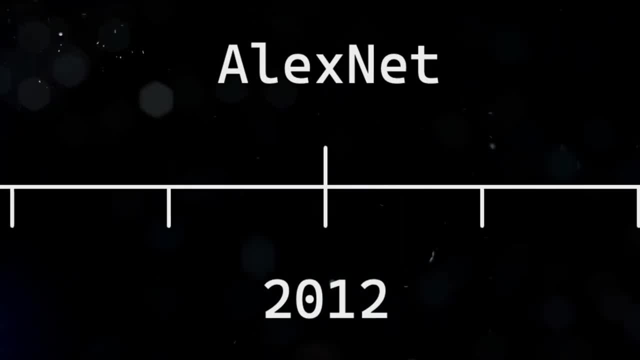 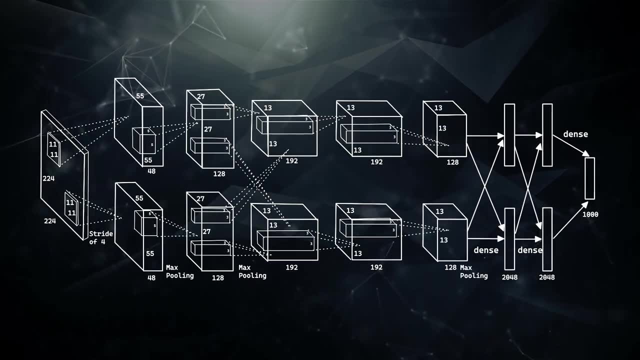 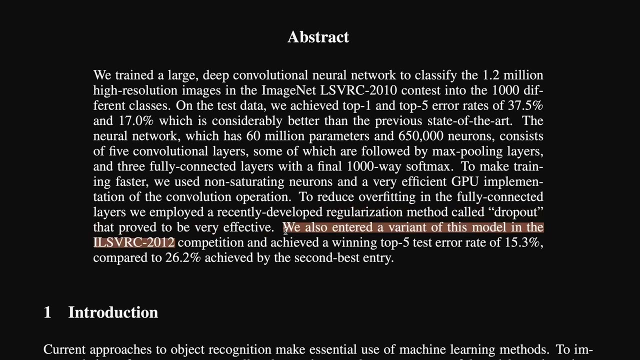 And that is where we got AlexNet. So AlexNet is the deep CNN that kick-started the era of deep learning, And that was back in October 2012.. The catalyst of this was AlexNet winning the ImageNet competition And, in fact, AlexNet can actually be seen. 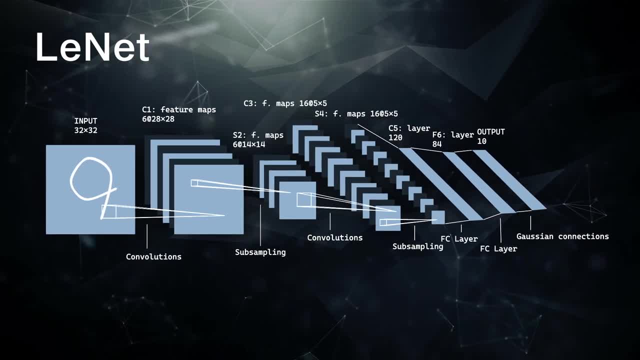 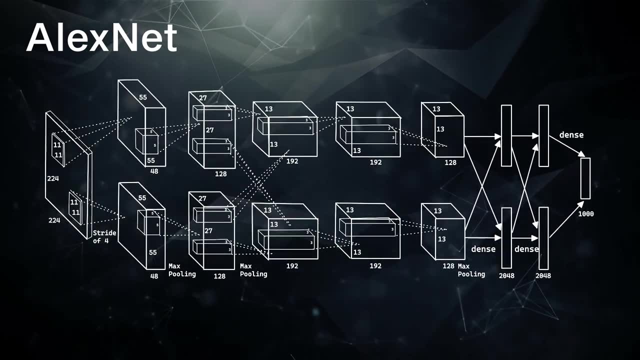 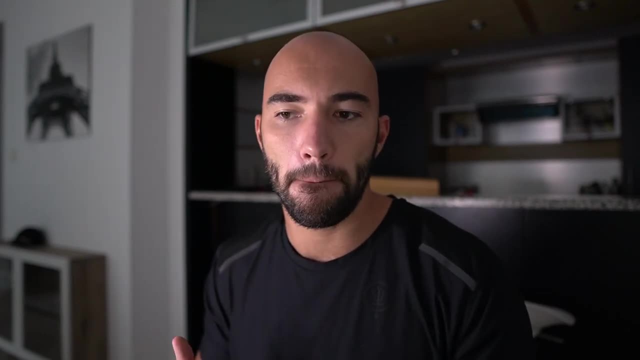 as a continuation of LeanNet. It uses a very similar architecture, but simply added more layers, training data and some safeguards against overfitting. And it was after AlexNet that the broader community of computer vision researchers began focusing their attention on building ever deeper models. 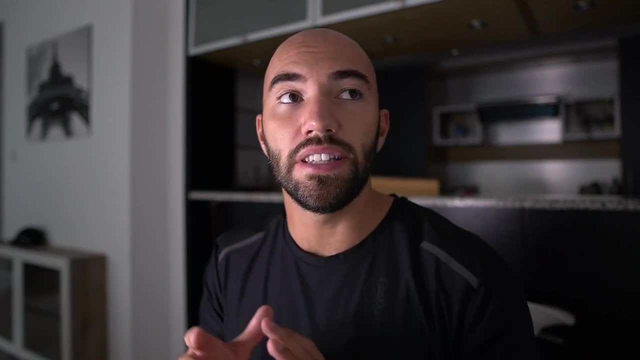 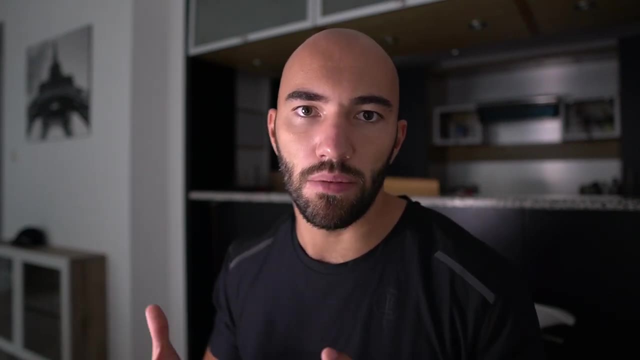 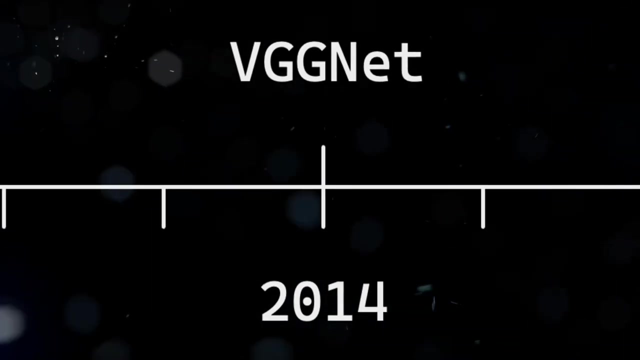 with really big data sets, And the following years after this basically saw many variations of AlexNet winning the ImageNet competition until we get to VGGNet Now. VGGNet came in 2014 and dethroned AlexNet as the winner of the ImageNet competition. 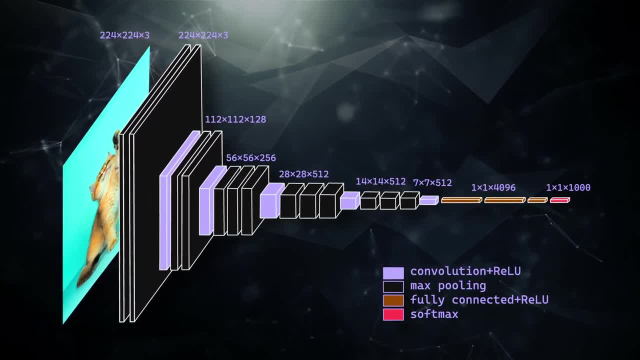 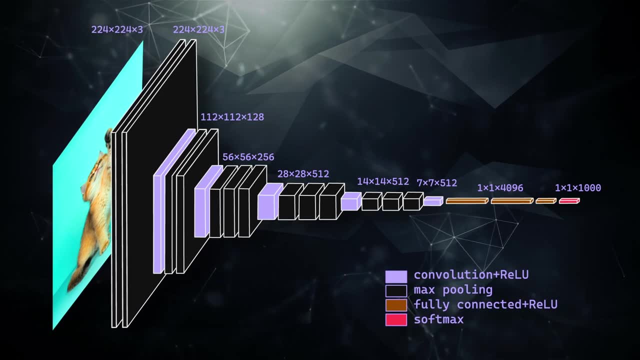 And there were a few different variations of this network developed, but we can already see that it's a much deeper network, But at its core it's still using the same, the same process of convolution layers, pooling layers and so on. 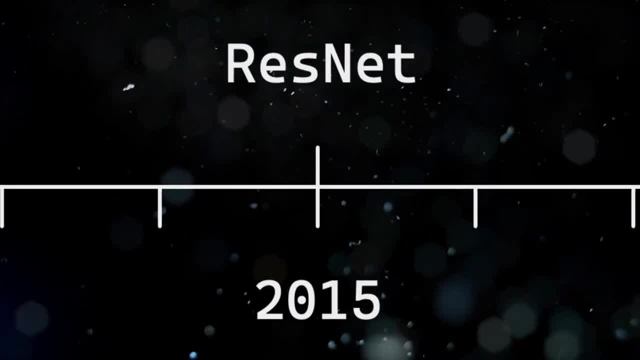 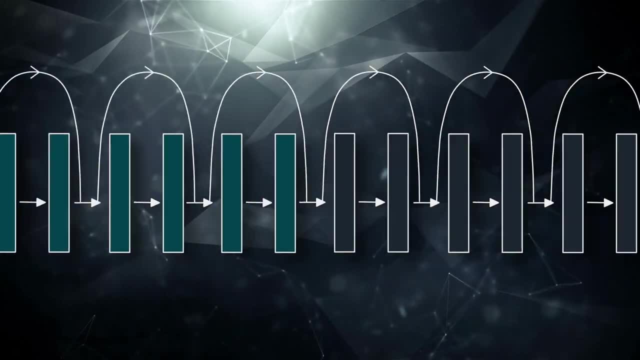 Moving on to 2015,, the next year, we saw the introduction of ResNet. Now, ResNet introduced even deeper networks than ever before. The first of those contained 34 layers And since then, 50 plus layer ResNet models. 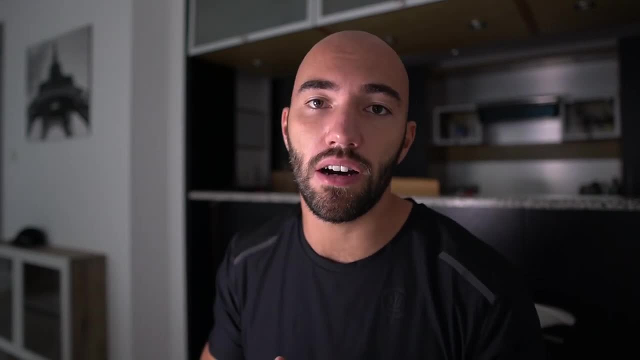 have been developed and still hold some of the state of the art results on many computer vision benchmarks. Now, beyond adding more layers, ResNet was actually very much inspired by VGGNet, but added smaller filters and a generally less complex network architecture. 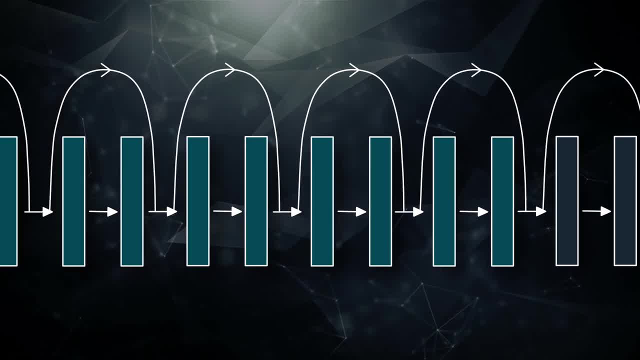 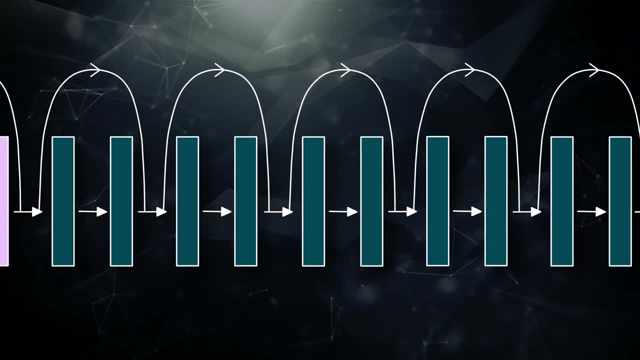 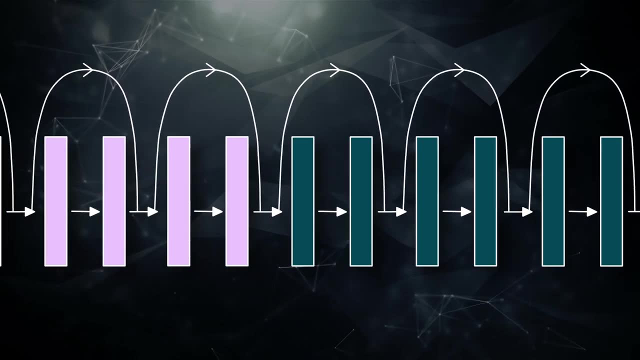 Another thing, which is why it's called the residual network, eg ResNet, is they added these shortcut connections between layers And this was to avoid the loss of information over many layers with the greater depth of ResNet. So adding these 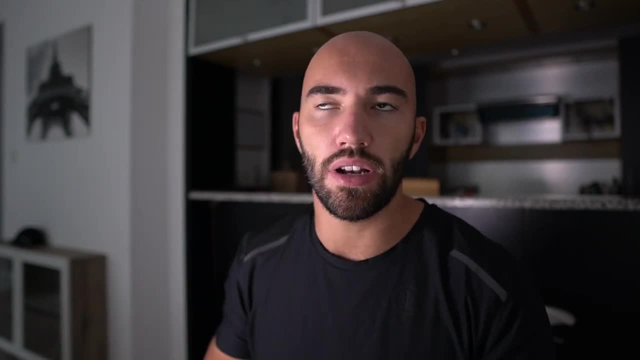 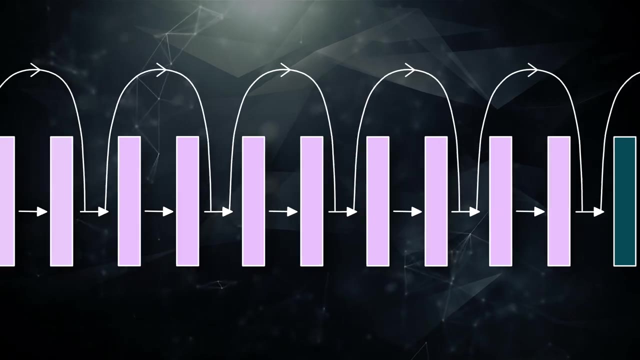 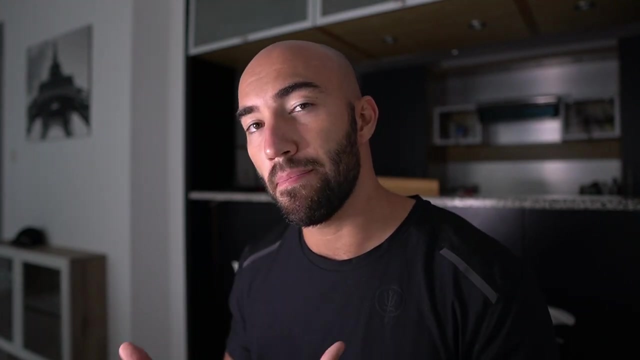 shortcuts. all these residual connections just allowed information to be maintained over a longer distance, which was very much required with this deeper network size. Now, I think that's enough for understanding convolutional neural networks. What I want to do now is actually look at how to implement. 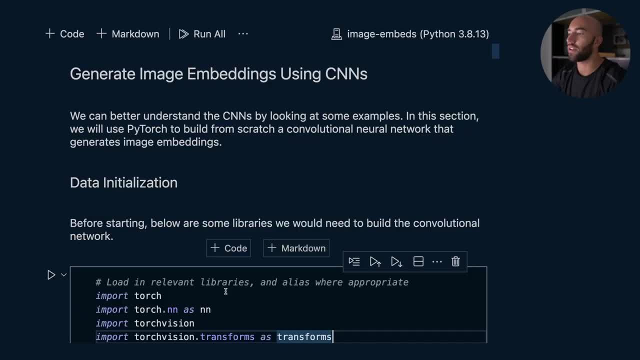 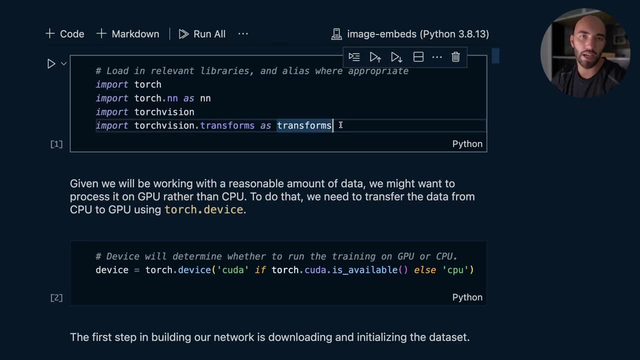 convolutional neural networks and use them in classification. So we're going to go through this notebook example here. You can find this notebook in the video description and you'll be able to open that in Colab if you prefer. you can actually download the file as well. 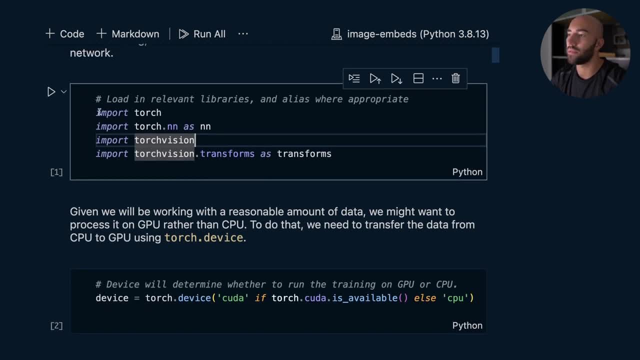 We're first going to just load in the relevant libraries. So we have PyTorch here and TorchVision. I'm going to be using these transforms a lot, So we'll just also import them, as transforms make it a little bit easier. 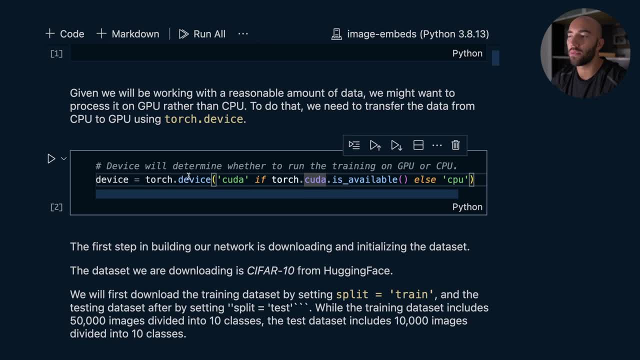 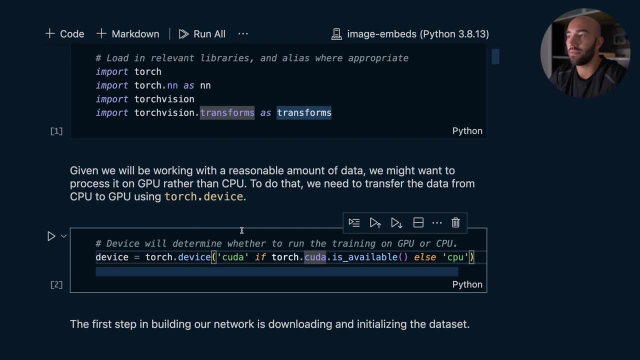 Now we're going to be working with a fair bit of data, So what is usually pretty helpful to do is switch from CPU to GPU if you have it available. We don't always have it available, but it can be useful if you do have it. 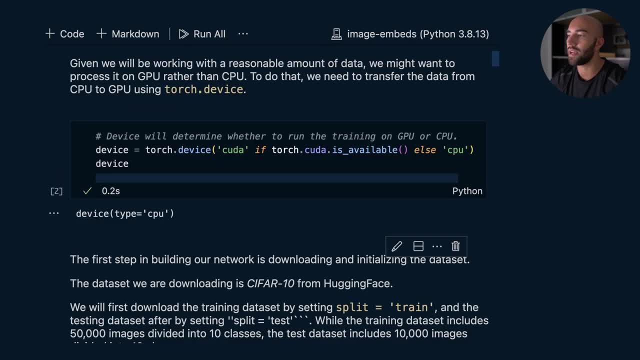 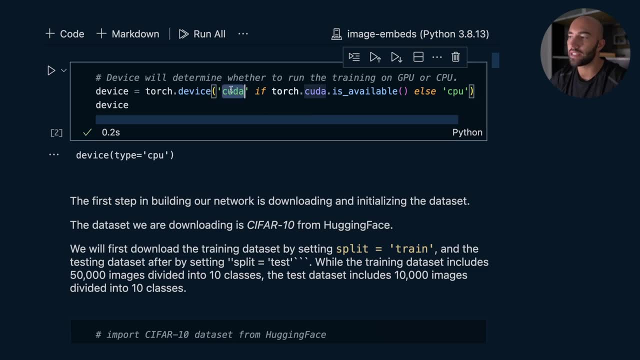 And you can just check what you have like. so So for me I'm on MacBook right now, so I only have CPU, But if you're working on Colab, this should show up as CUDA. Now, as usual, our first task. 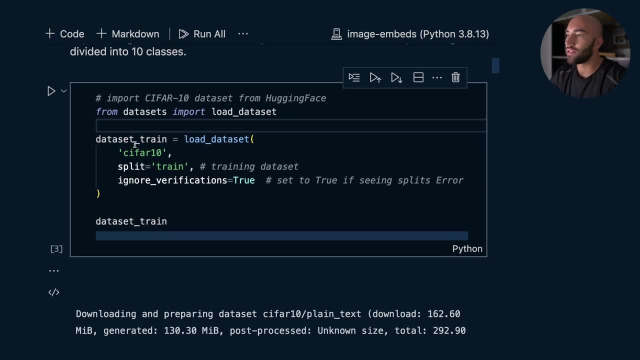 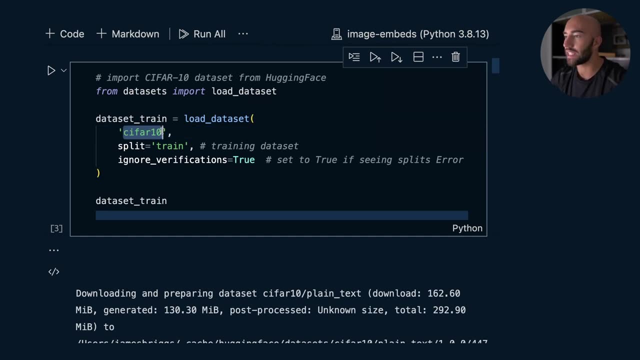 is going to be data pre-processing, So we first need to download our dataset. We're going to be using the CIFAR-10 dataset, which is a very popular image classification dataset. Download that and we will see that it contains 50,000 items. 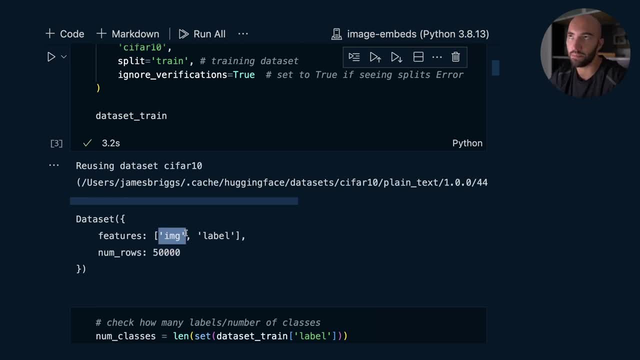 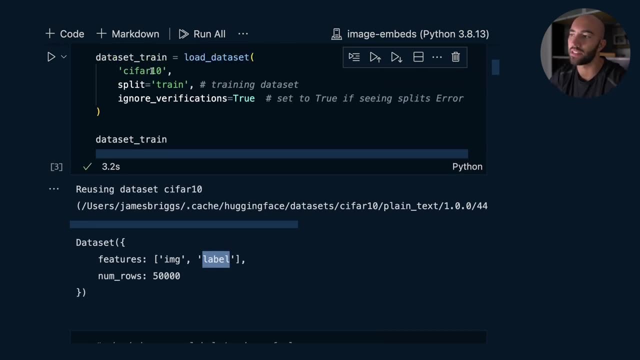 and within that we have images which are just Python, pill image, objects and the labels of which there are 10 unique labels within the dataset, hence why it's called CIFAR-10.. And we can confirm that here, So we see that we have 10 of these. 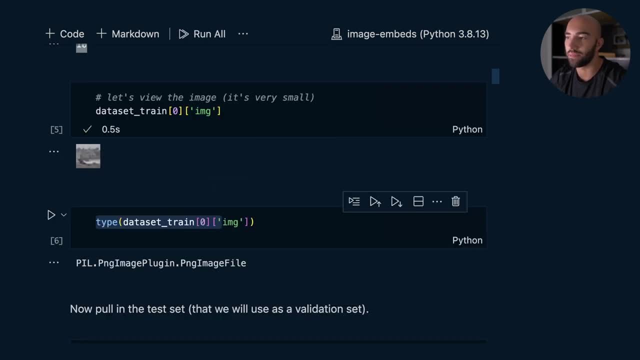 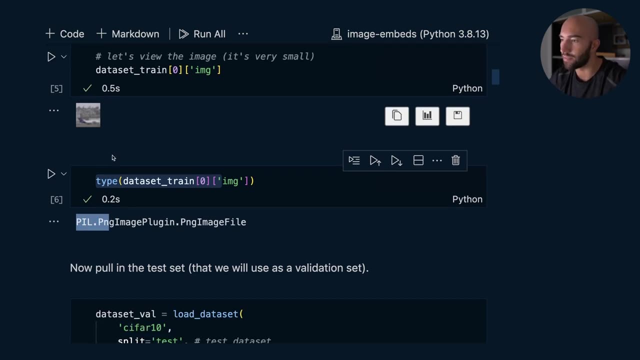 and then we can also view the images, but they are very small. We can also see that they are Python pill objects here. So this is, I think, a plane, but yeah, it's very small. So we're going to be training the model. 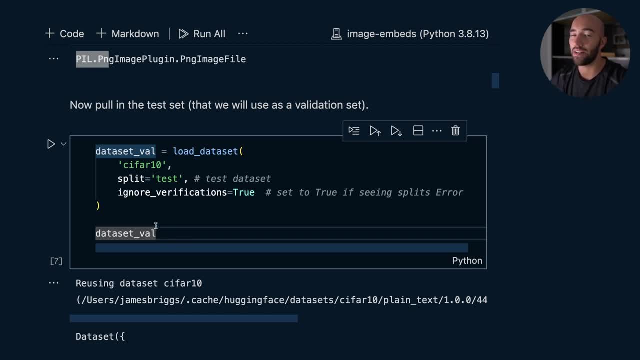 and while we're training, we also want to pull in another dataset that is independent to the training dataset, that we can use as a validation or test set later on. We're going to be using this test dataset actually as a validation dataset. 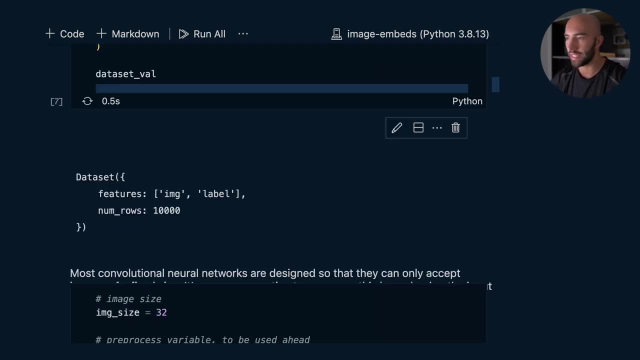 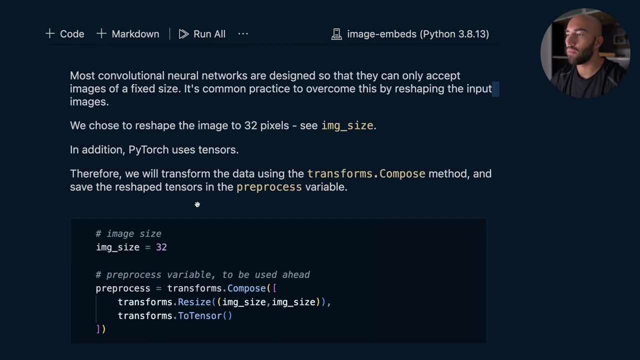 So we're going to be checking our model performance on this data during the training process. You can see that we have a smaller number of items in here. It's 10,000 from 50,000.. Now, most convolution: neural networks. 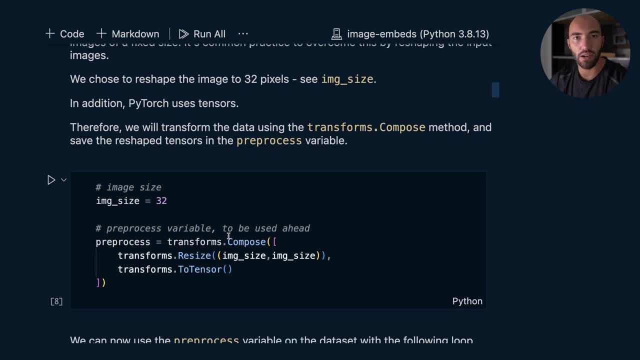 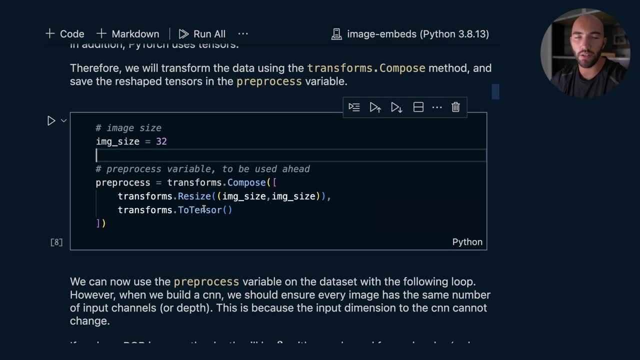 are designed to only accept a certain size of images. In the case that we are going to use, we're going to use a 32 image input. We can modify that based on the model architecture, but the model architecture that we're going to be using later. 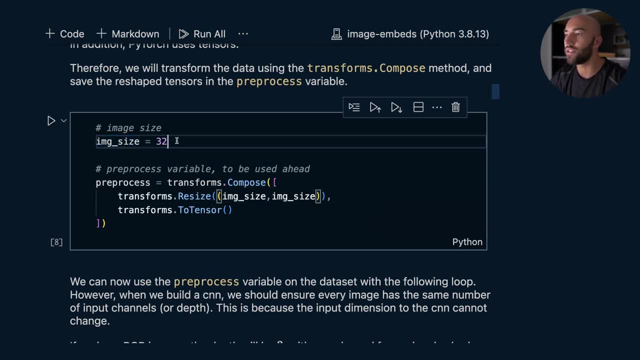 accepts this 32 by 32 image size. So what we need to do is we can set the image size here and then we can use transforms resize to resize the image into whatever we put in here- so 32 pixels, And then this transforms to tensor. 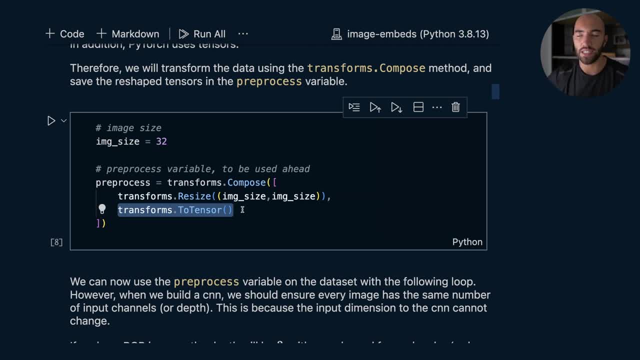 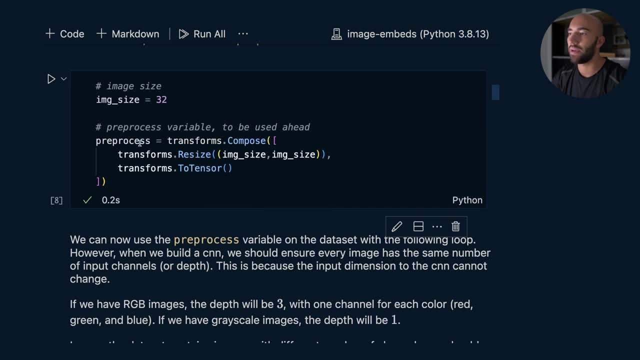 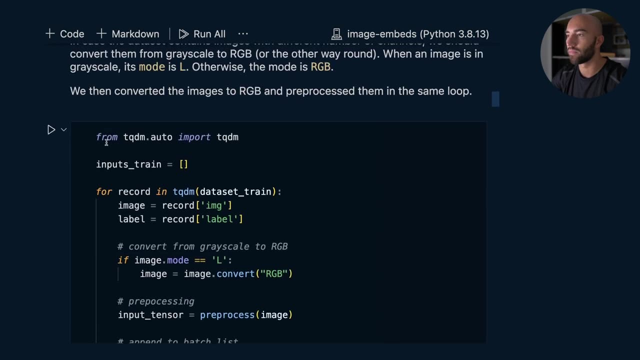 is just to convert our image, our pill image, object, into a tensor in which we can then feed into our model later on. So run this and basically we can just run preprocess on our images and that will run this transformation pipeline across them. 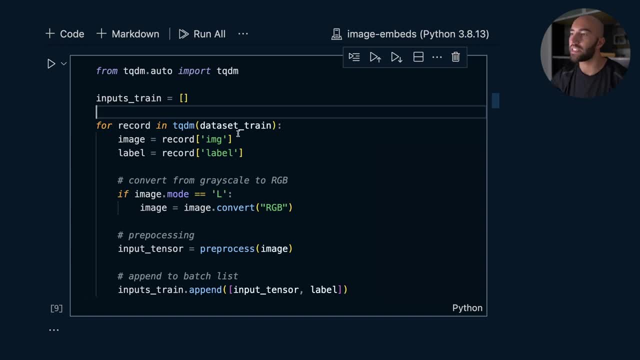 Now there are a few things to consider when we're doing this. The first is: okay, we're gonna be iterating through everything we need to extract the image and its respective label, One thing we need to consider with this image dataset in particular. 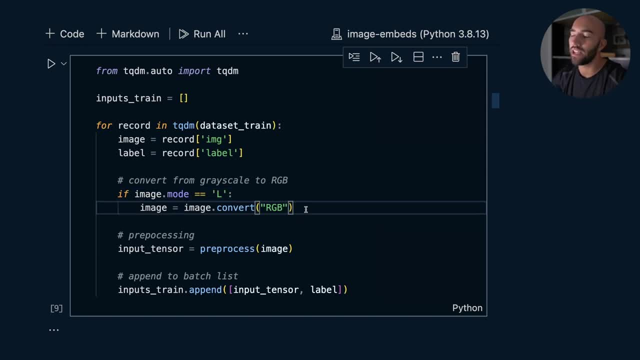 but other image datasets as well, is we only want one image format, So I want to have RGB images, so images with red, green and blue color channels. A few images in this dataset are actually just grayscale, so they have a single color channel. 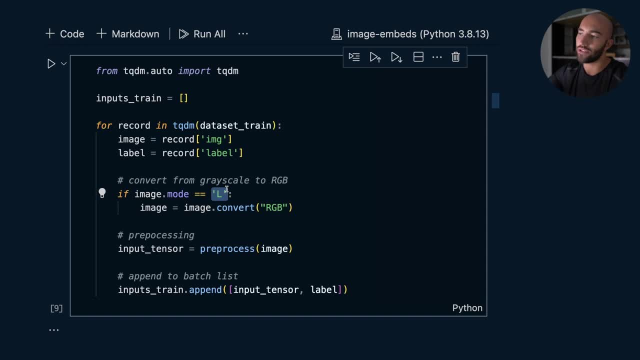 Now, we're not going to colorize it or anything like that. We're actually just going to copy those single color channels into three color channels and it will still appear as a black and white, grayscale image, but we at least have those three color channels. 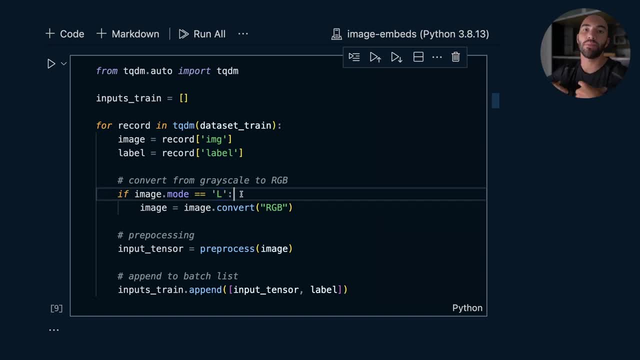 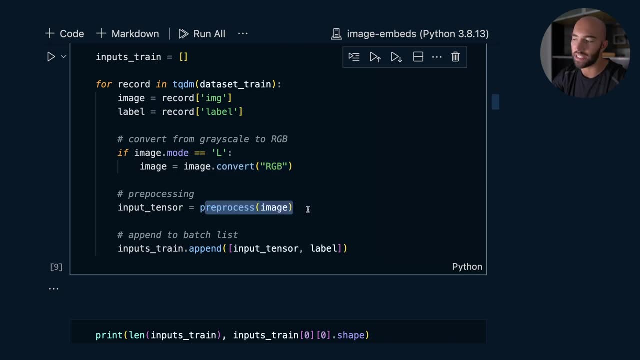 which means we can pass that directly into our model, which expects image arrays with three color channels. So we do that using image convert here, and then we pre-process everything and then we append all of that to our inputs. Okay, now we'll just take a moment. it's pretty quick. 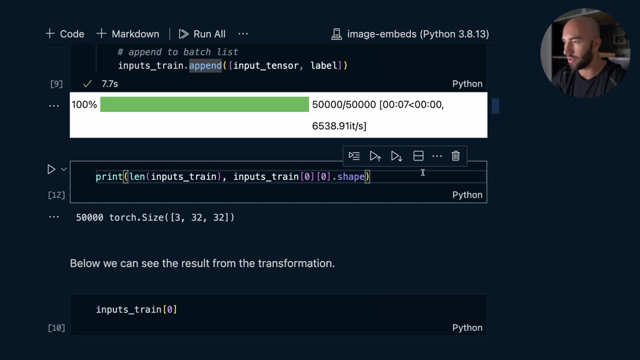 Now let's have a look at one of those images. So we run this and we can see that we have 50,000 of these modified images in our training set, and each one of those is a three by 32 by 32 tensor. 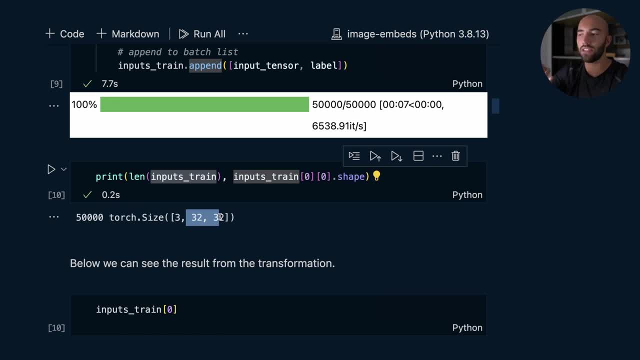 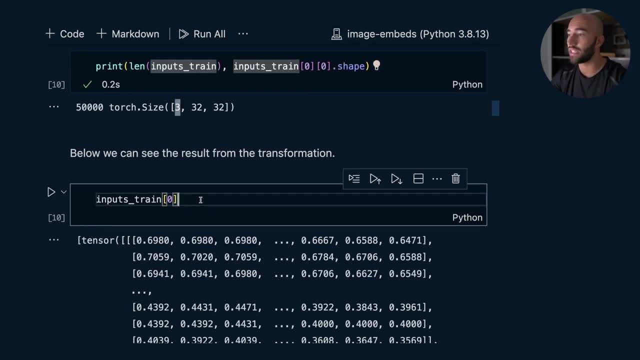 Now 32 by 32 is the actual pixels in the image and the three is the number of color channels- red, green and blue- And we can see the result from this transformation here. so this is just a tensor. One thing to note here is that all these values 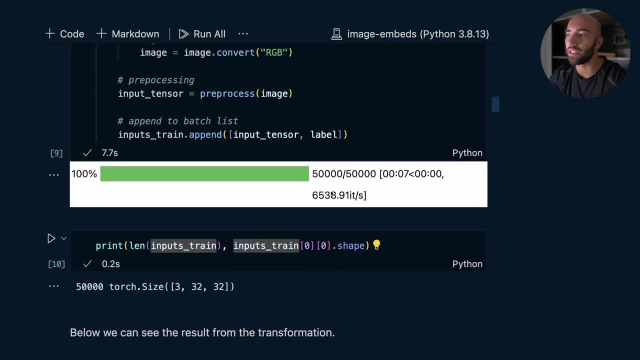 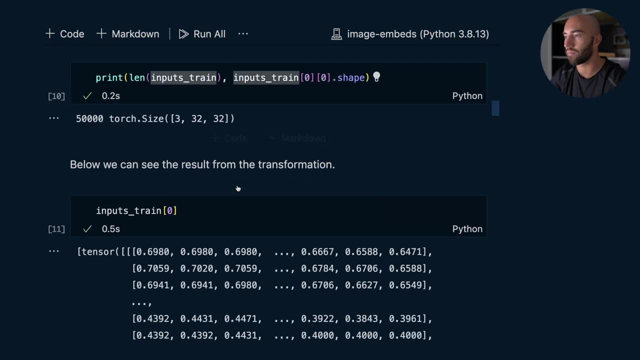 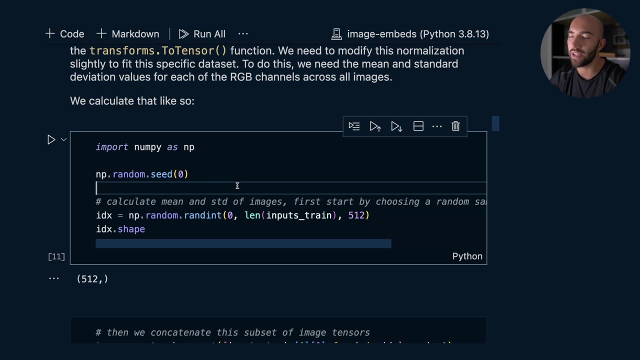 have been normalized to between zero and one. That was actually done pre-processing pipeline here with the transformsto tensor. Okay, so, moving on, one thing that we should do is calculate the mean and standard deviation of images so that we can modify the normalization. 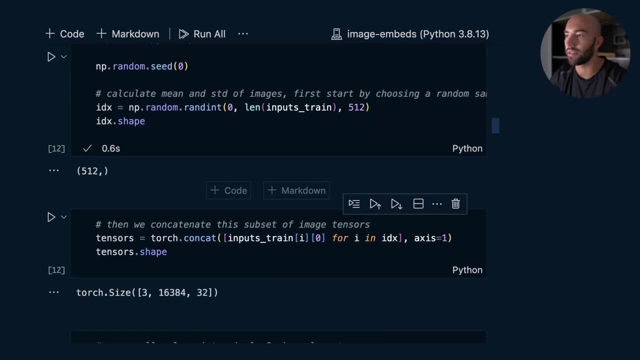 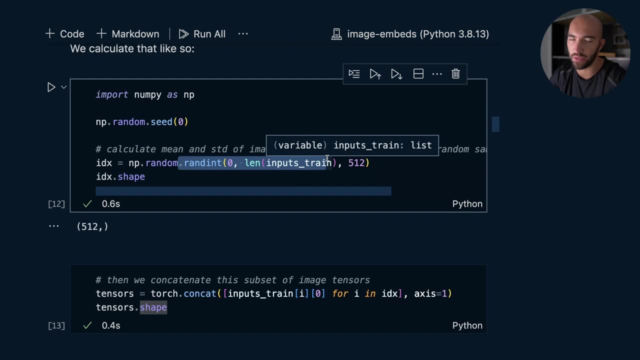 to better fit our set of images. So to do that, we would do this, creating a big list of all of our images, And this is just a small subset of those that we pulled from here. So this is like we're sampling a smaller portion of those. 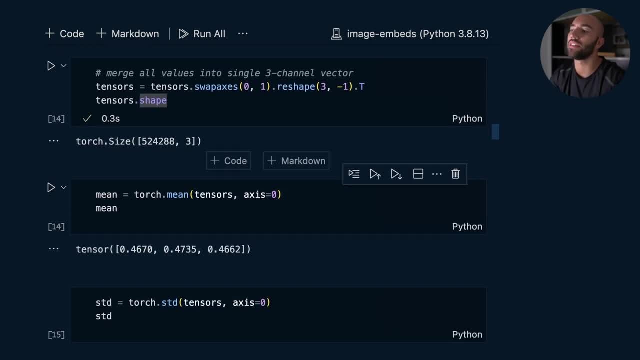 Otherwise this just takes a bit longer. We're merging all these into a single three-channel vector. So you can see, here we're just kind of merging all those images into a massive one, single big image, And then we just want to calculate the mean. 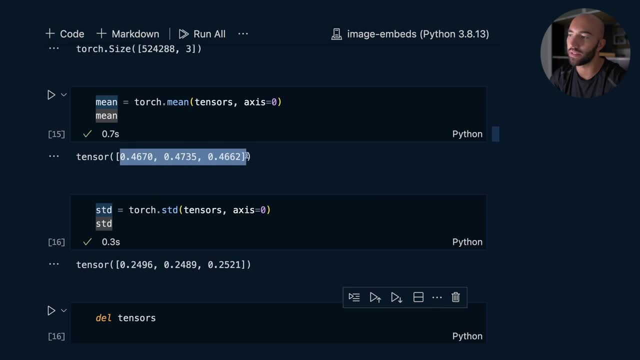 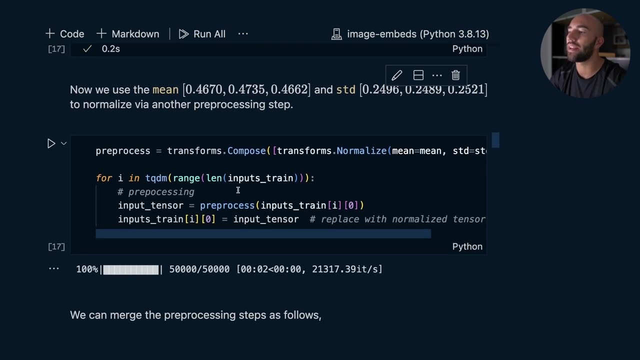 and the standard deviation for each one of those color channels. Okay, so we get these values and these values. Now we don't need those tensors anymore and they take a bit of space, so I'm going to remove them. And then what we do is we just modify. 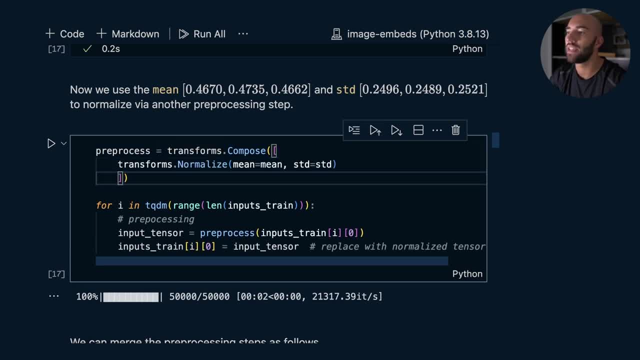 that normalize here, okay. So now we're just normalizing all of the tensors with this additional step here, okay? So we've pre-processed that and we apply that to the existing tensors. Run that, okay, and that's done. 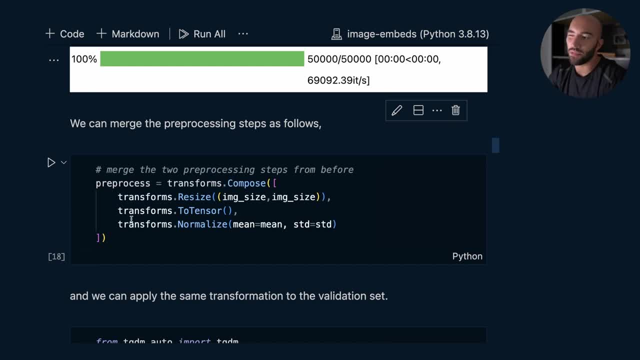 But obviously, when we're doing all of this in one go, we would probably want to do this, So we put all of them into a single pre-processing pipeline so we're able to resize the two tensor and then normalize following that, And we'll actually use that on the validation set. 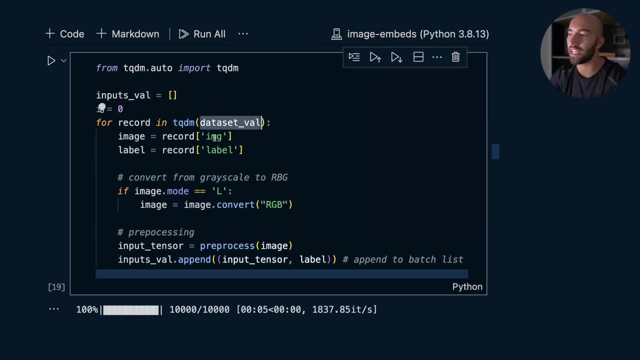 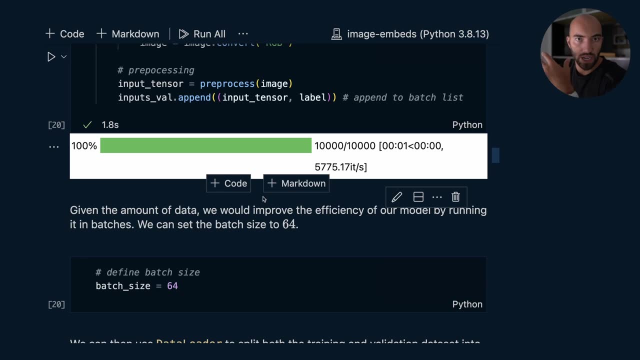 So here is our validation set, and we'll just rerun that same thing as before, but obviously this time we have that normalization step in there as well. Now, when we're training a model, we are probably going to want to do it in batches. 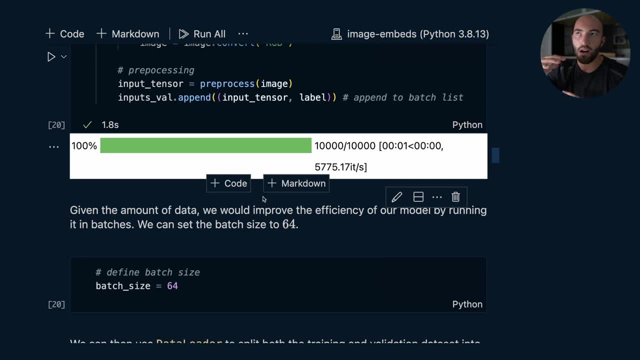 So we want to pass through a batch of input data at any one time into our model, So we're passing, rather than passing, a single image at a time through everything, we're passing everything through in batches of, in this example, 64.. 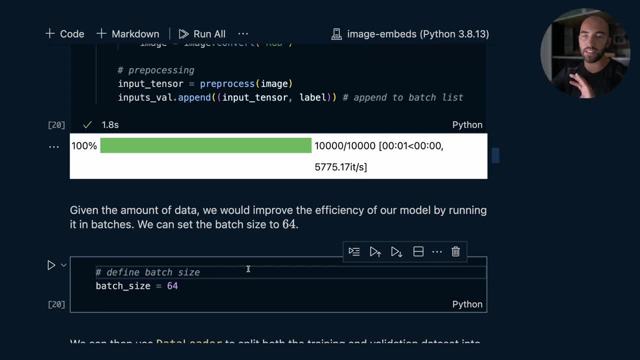 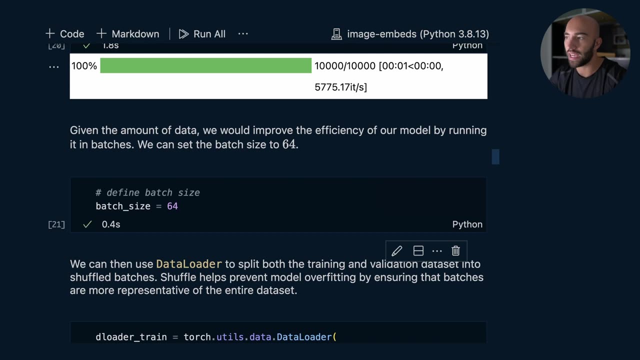 And this is because neural networks can be paralyzed, and that allows us to take advantage of paralyzation, which means we're performing many calculations across all of these different images in a single batch in parallel, rather than one after the other, which means everything will be much faster. 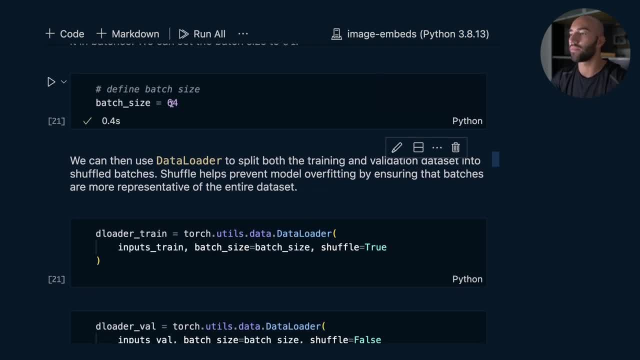 Now to prepare everything, we need to load everything into our data loader. So this is going to handle the loading of data into our model. We have the batch size here. We're also shuffling everything so that we don't have like the same set of images. 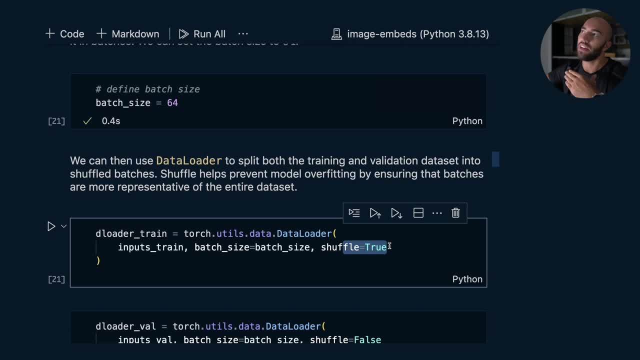 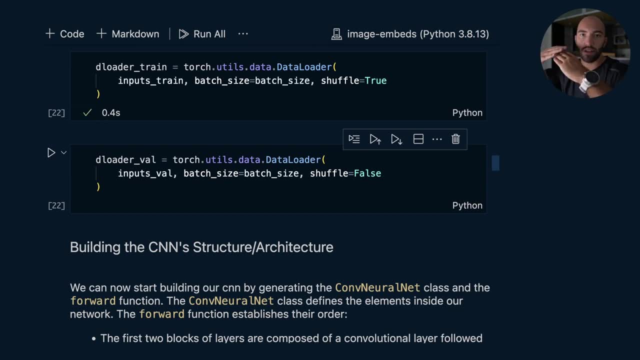 if they're not shuffled already within the dataset so that we don't have the same set of images all covering a single batch. We want every single batch to be as representative of the full dataset as possible. Now we initialize data load for both the validation and the training set. 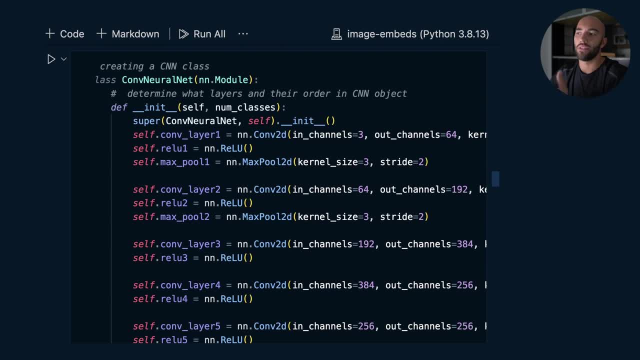 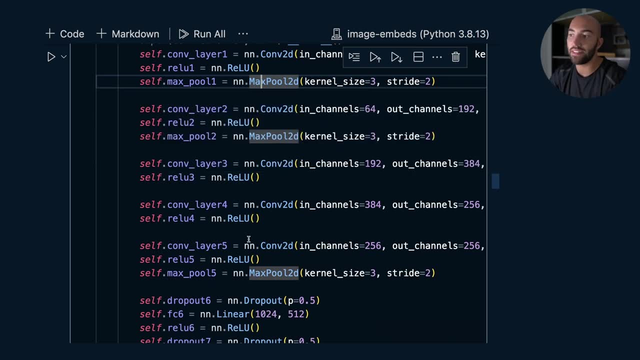 And then what we're going to do is actually build our convolutional neural network. Now, it's pretty big, but that's just thanks to the number, the depth of the network In reality, if we compare it to a lot of the networks. 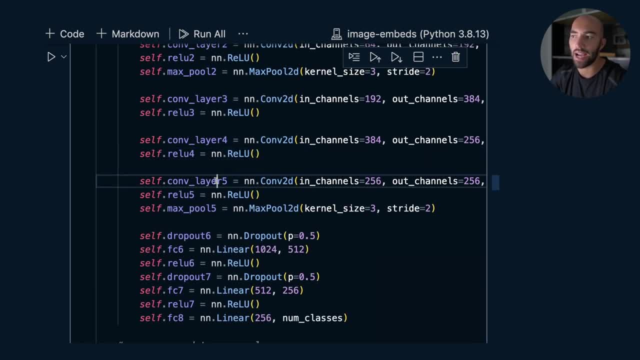 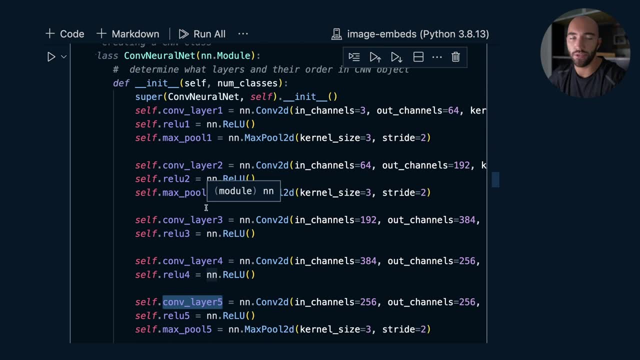 we looked at before, it's not actually that deep. We only have five convolutional layers here and then a few other things, But you should note that there are a few things that you might recognize from before. We have the convolutional layer, followed by radio activation layer. 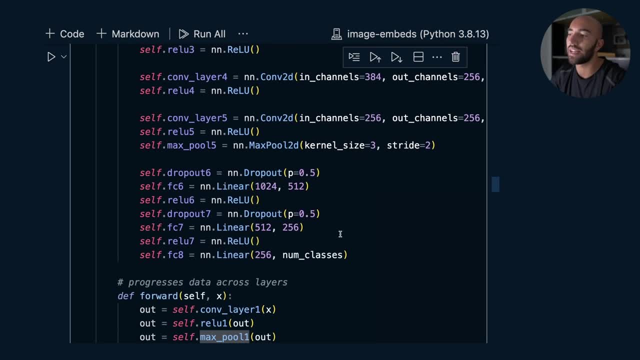 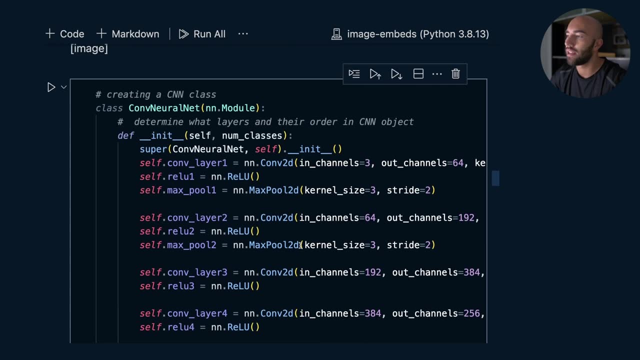 followed by max pooling layer, and we do that several times, And then at the end here we have our fully connected layers. We have a few of those in order to get our predictions. Now, things to note here is that we have a number of input channels here. 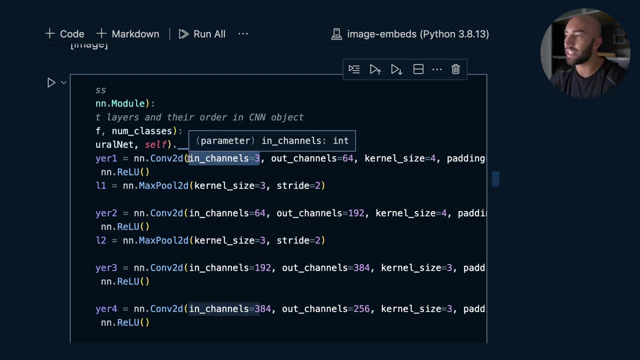 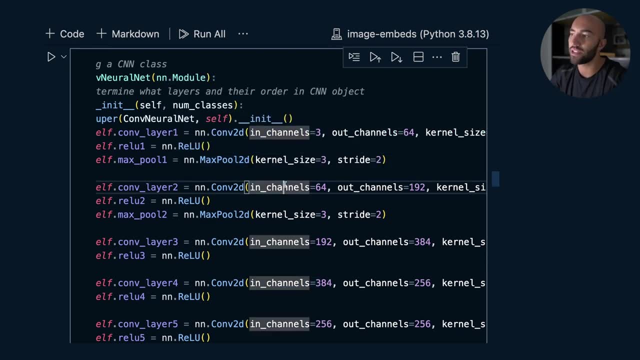 This must align to the number of input color channels that we're expecting. Our inputs will be identified based on the first set of input data that we throw into our model, So that will be 32 by 32.. And this first convolution layer is going to go. 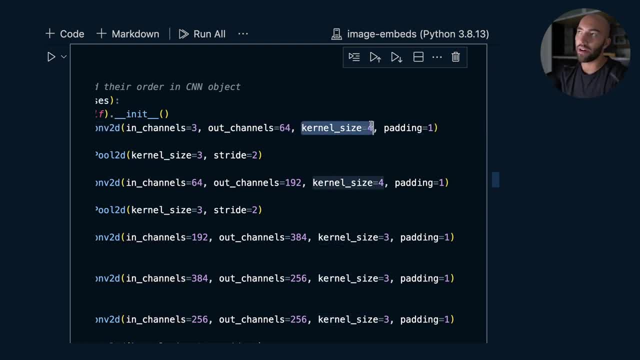 and it's going to go to the first set of input data that we throw into our model, So that will be 32 by 32.. Over that, 32 by 32 images with a kernels, or a window of four by four images and go through that. 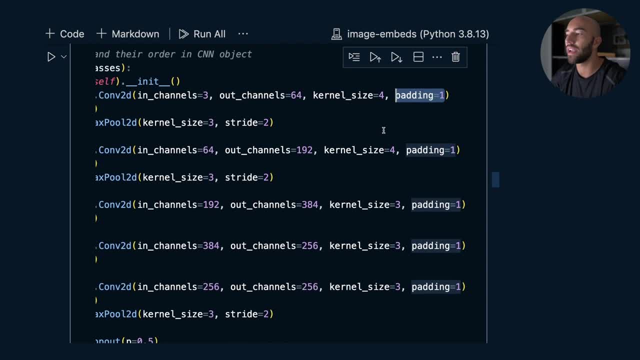 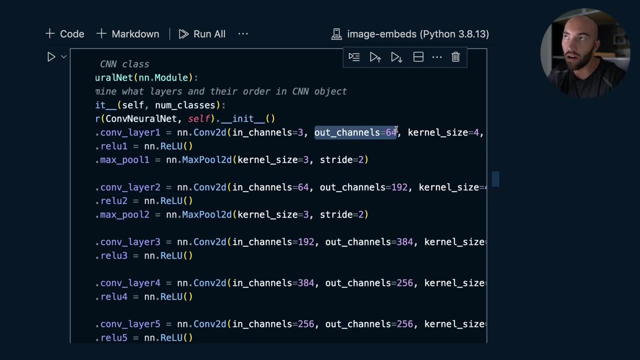 We'll also add some padding to reduce the amount compression And we do that throughout the network. Now, other thing actually to note is the number of output channels is the depth of the array. So the depth initially is three color channels. The depth from the output of that is actually 64.. 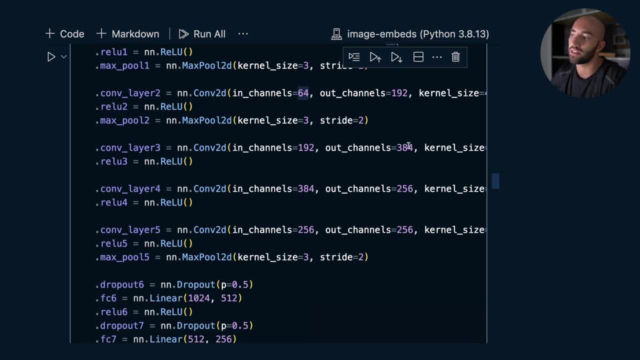 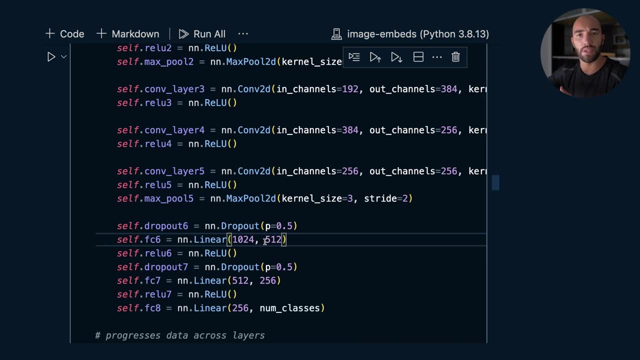 And that gets deeper and deeper as we go through, before we start decreasing that, Before we start decreasing that, As we're going towards the end of the model, And then, at the end, here we're just performing transformations from our 3D convolution layers. 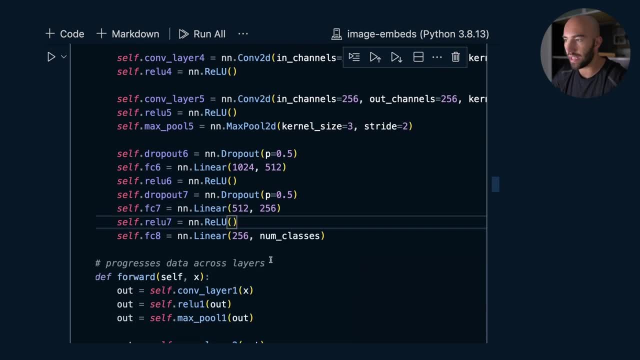 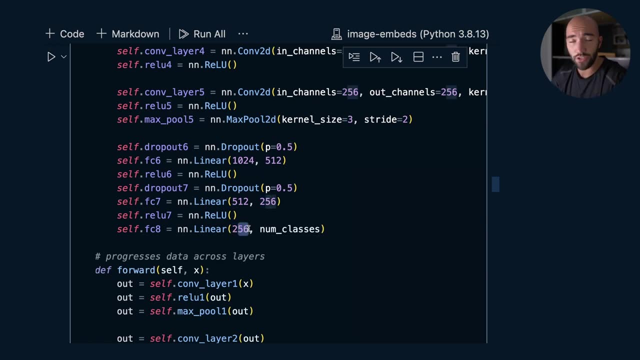 into the fully connected layers at the end there And the final output. so this is our final layer. The input to that layer is 256 activations or nodes, And the output is the number of classes, which is 10.. Then what we do? so, that's defining the structure. 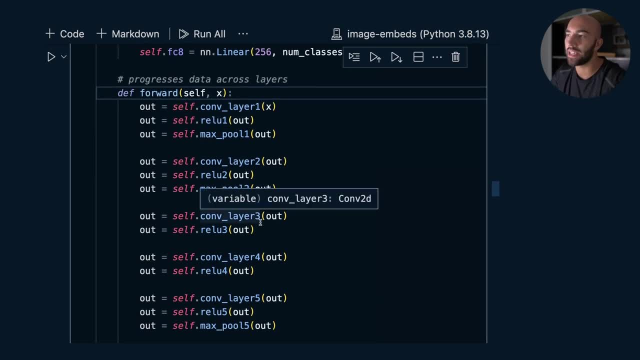 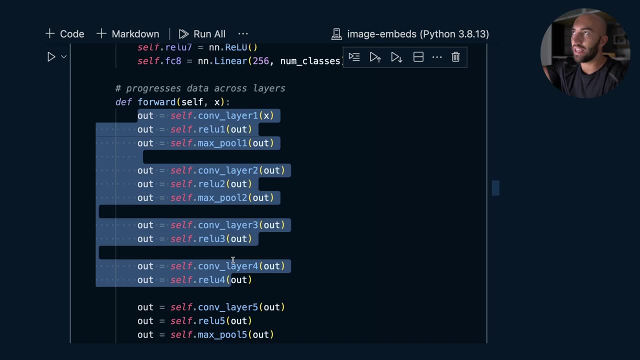 of our convolutional neural network, Then what we do so, that's defining the structure of our convolutional neural network. The next bit here is the forward step throughout, So it's identifying or it's defining the process that we move through each one of these layers. 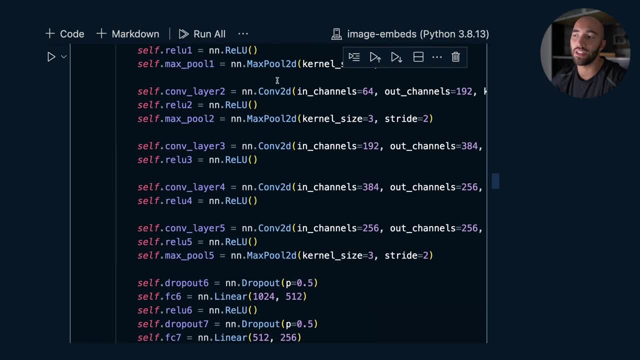 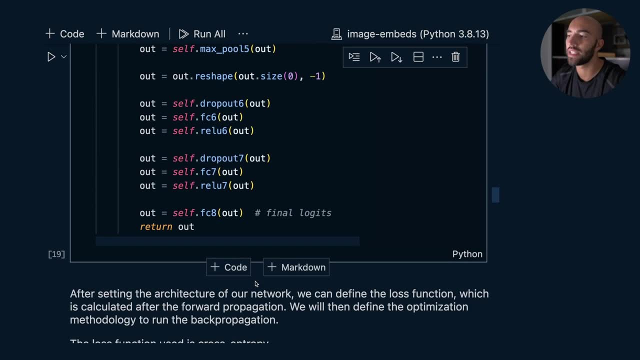 the order that each one of them is used, Because we can actually define all of these in any order we want, but it's actually here that the order is defined, So we go through that. We get to here, which is our final output. 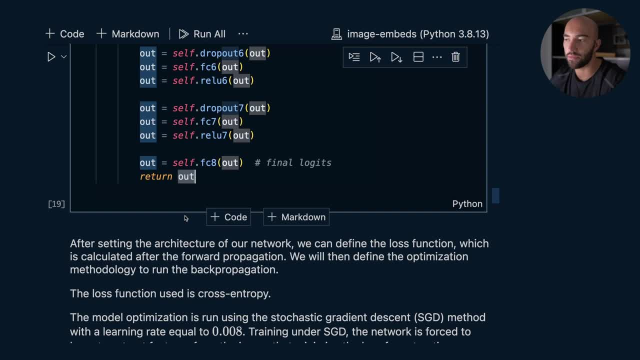 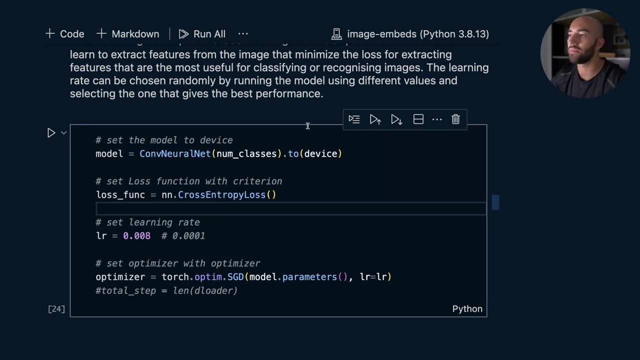 And that is how convolutional neural network And that is how convolutional neural network, that is how we define it. and then we come down and we move on to setting everything up for training. So we want to move it to our device if we're using a. 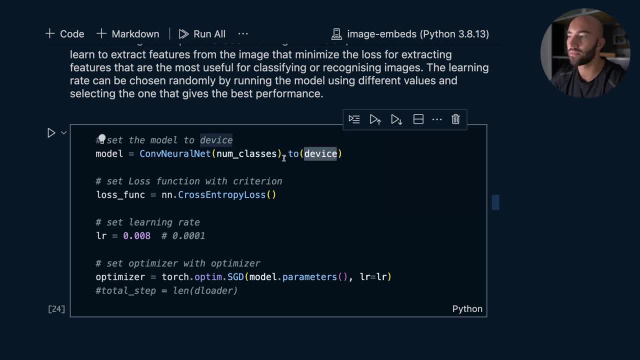 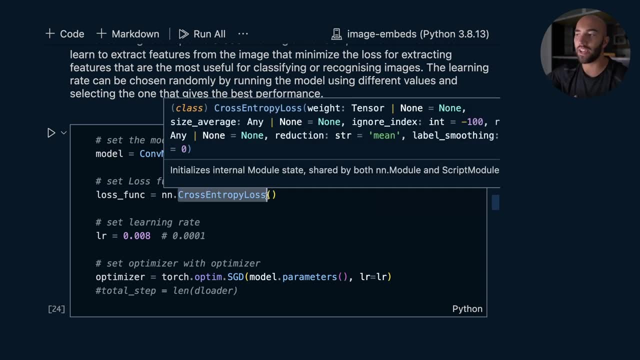 CUDA enabled GPU, otherwise it'll just stay on the CPU. We want to set the loss function. we're going to be using cross entropy loss. This is used when we have a classification task, like what we do here. Set learning rate so 0.008 and we're. 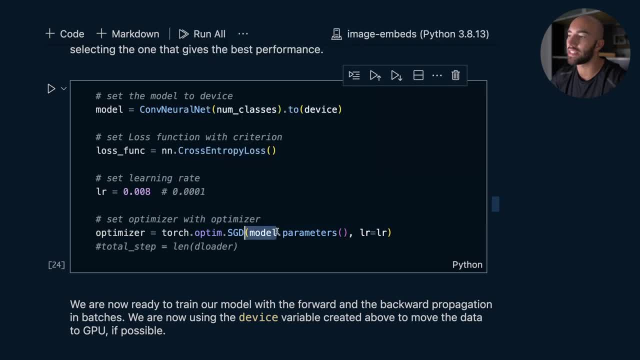 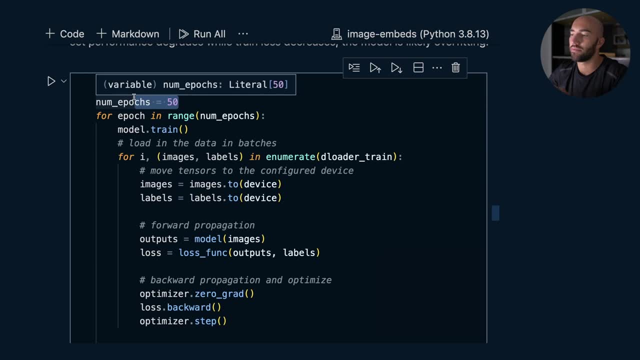 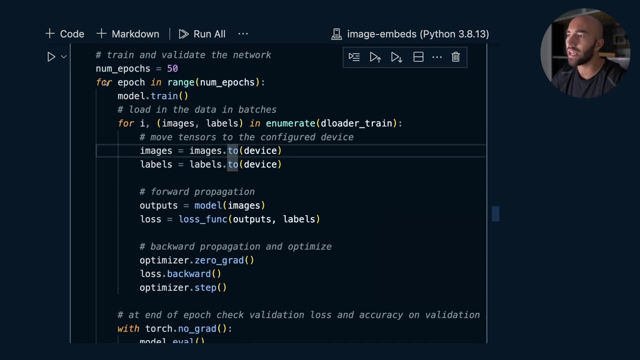 going to use stochastic gradient descent here as our optimizer Moving on. we would go down to here. we train it for about 50 epochs here. you can less or more, depending on what you're seeing on your end during the training. It doesn't take too long to run anyway, and then we run through the training, So we go through. 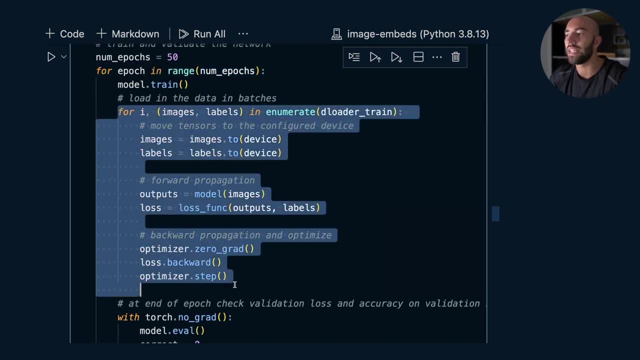 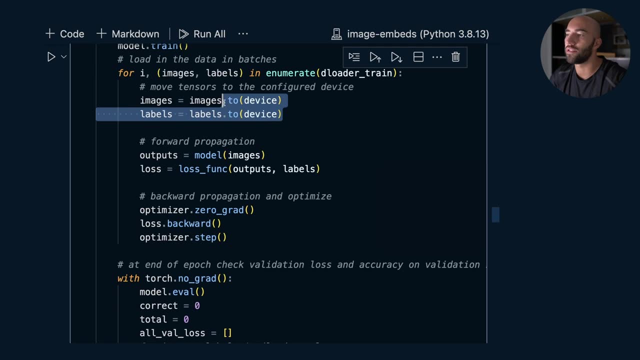 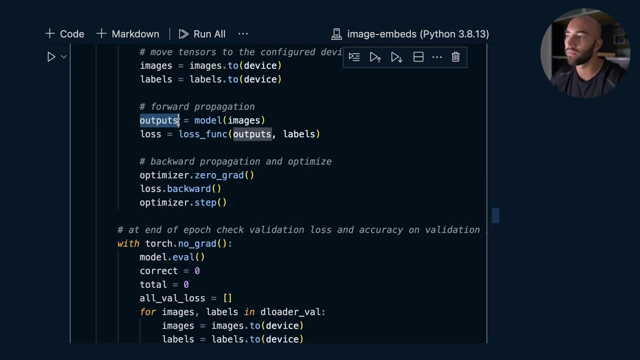 these 50 epochs and within each epoch we run through the entire data set. We load that from the training data Loader, aprender. we move those to the GPU. if it is available. we do the forward propagation from here. we get our output logits, so that is the, the final output predictions, and then from there we calculate. 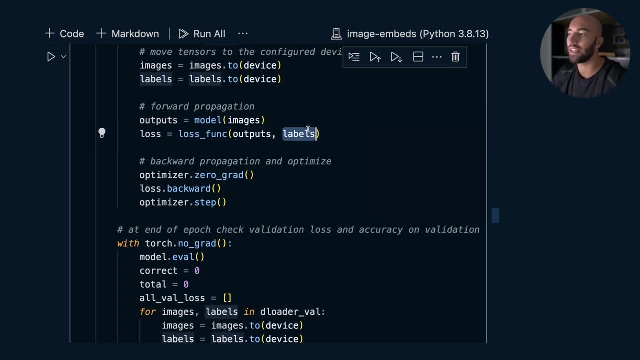 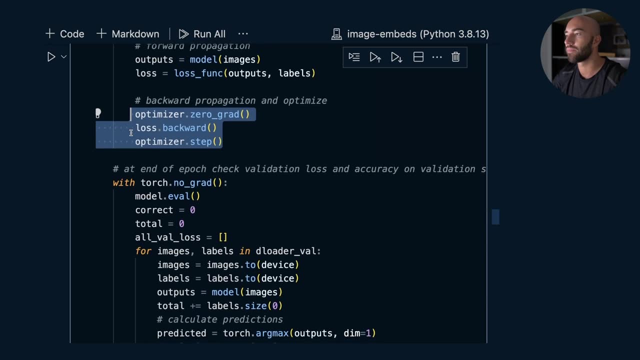 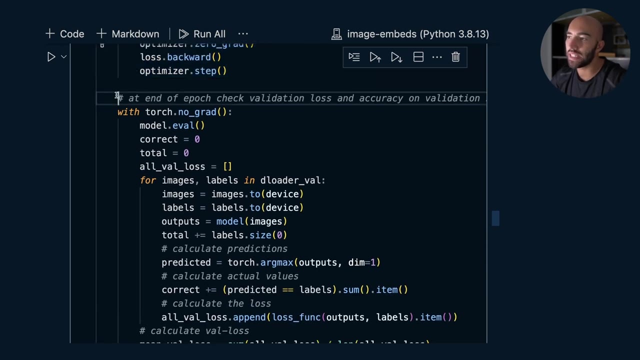 loss function between the predicted values and the true values. from there we optimize the model, so we do a backward propagation step and that is the training step. that's all for the training, and then this bit here is another bit. so this is for our validation, so that we can actually 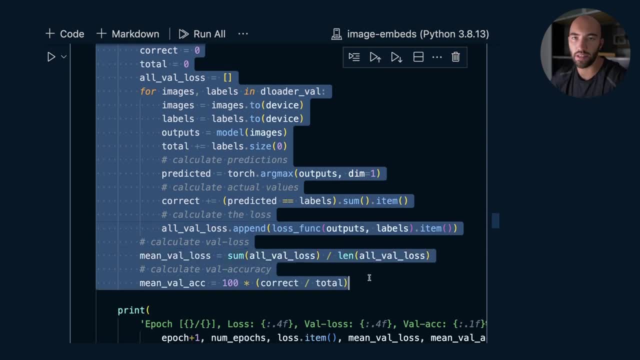 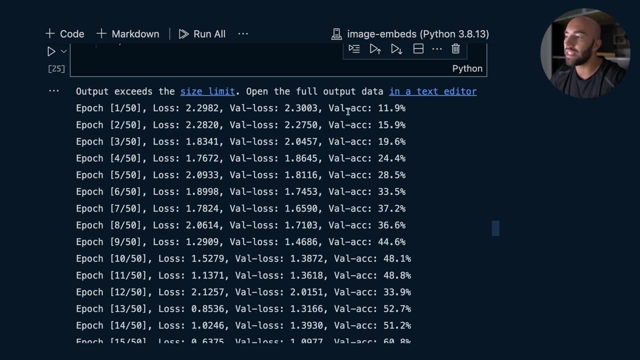 calculate the validation and just see that our model is not overfitting or anything over time and we will get something that looks like this. so important here is: if you see the loss decreasing and the validation loss increasing, that means that you're probably training for too many steps. 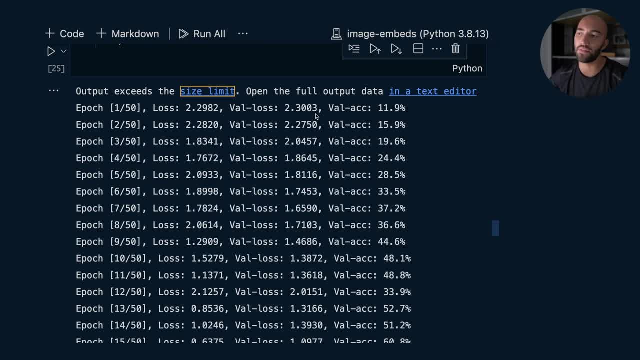 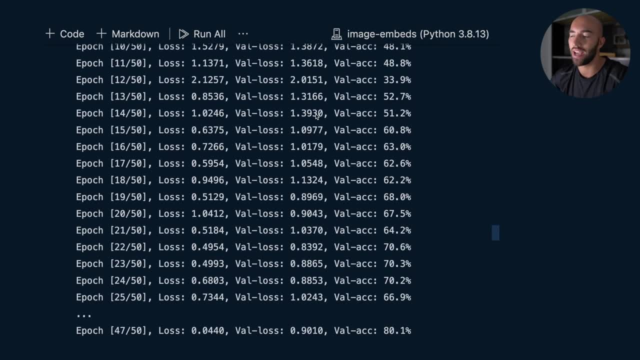 or your learning rate is too high and the model is overfitting to the training data. so in that case, just you can just just be wary and kind of stop doing that and either either train for less e-parks or train with a lower learning rate or with less layers, even okay. and then the final validation. I can see that we 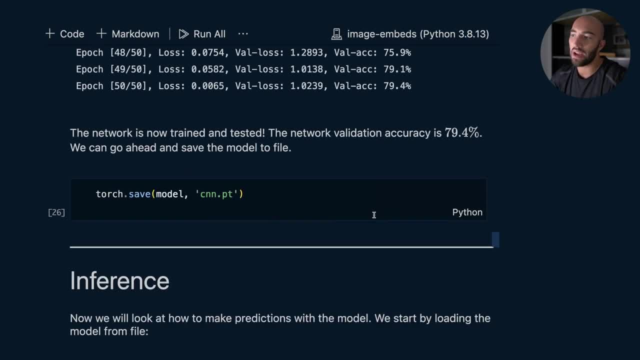 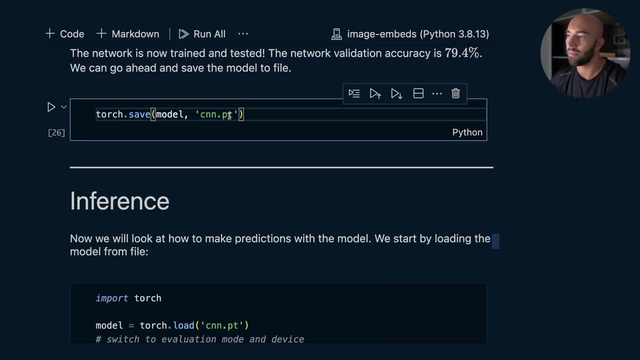 get near the end- here is around 80 percent- and we can then go ahead and save the model to a file like this. okay, so this is just CNN and the PyTorch weights file there. now, that is the, the training for the model. let's have a look at how we can use it for. 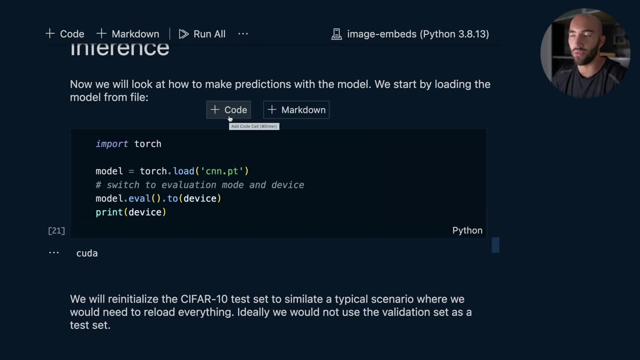 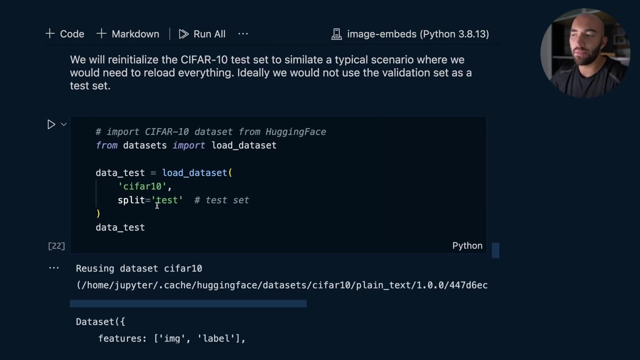 inference. so inference- by inference I mean making predictions- we would load the model, you know. if we didn't already have it in the notebook, we would make sure we switch it to evaluation mode and also move to device if we have CUDA node GPU- again pretending that we're not in the same notebook, we 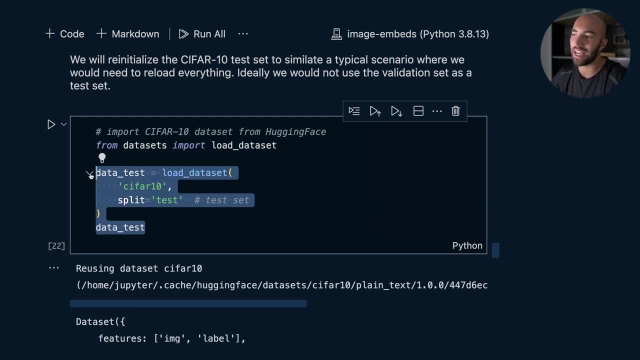 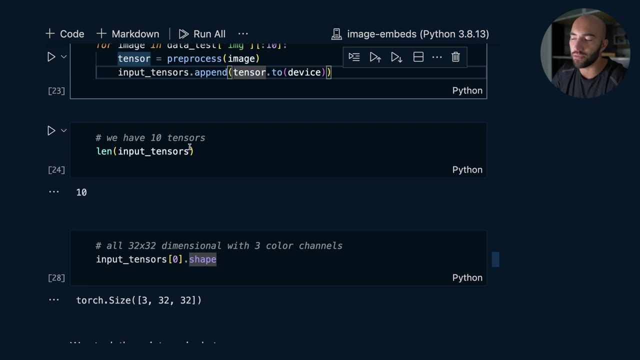 re-initialize the test set. so it's actually our validation set, but we're just using it for both in this example. of course, in real scenarios you should use a different data set for your validation and test set and come down here. we do the pre-processing that we sell before the 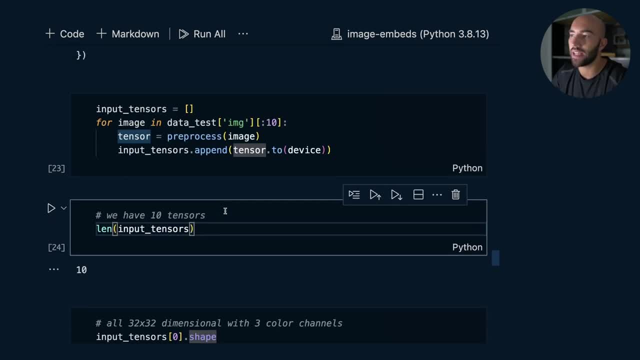 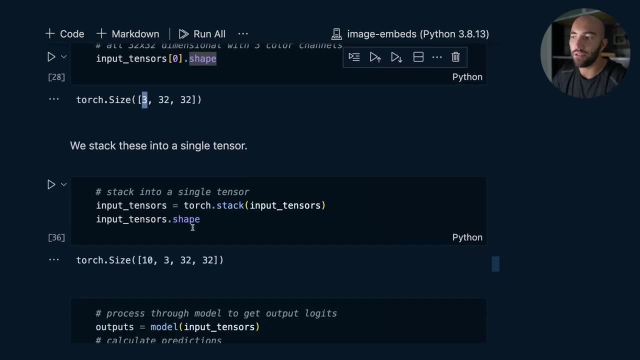 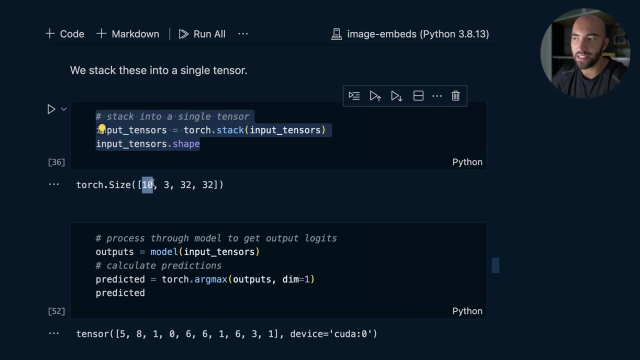 pre-processing pipeline, we check the number of tensors we have there. so we're just taking the first 10 as an example. all of those are the 3 by 32 by 32 that we saw before. cycle loads into a single tensor, so that we have basically 10 tensors or 10 image arrays. you can think of them like that. 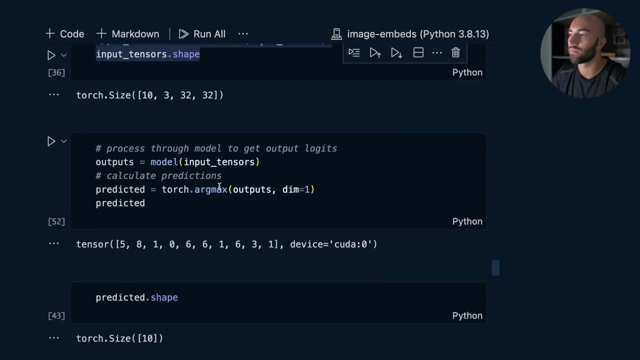 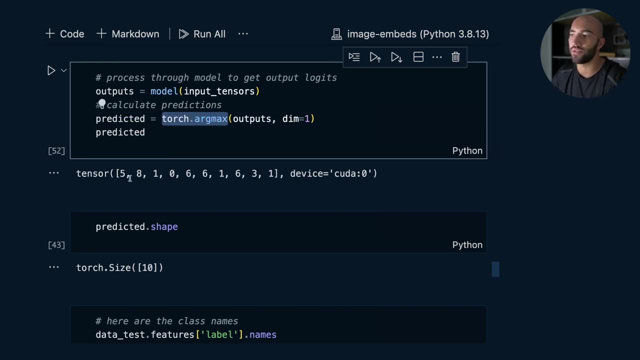 tensors and each one of those 32 by 32 pixels, process all of them through our model and then from there we can use the torch argmax function in order to find the value within the output logics that has the highest activation. and that is our prediction. okay, so in the first example position, 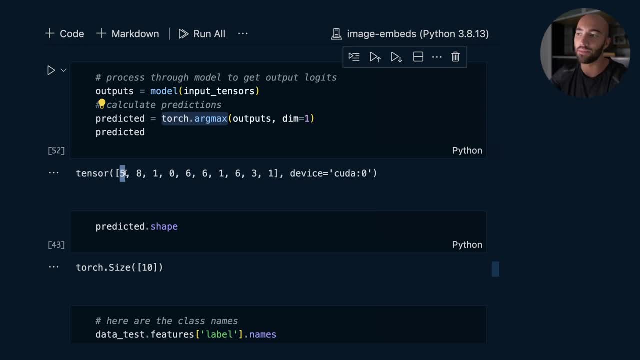 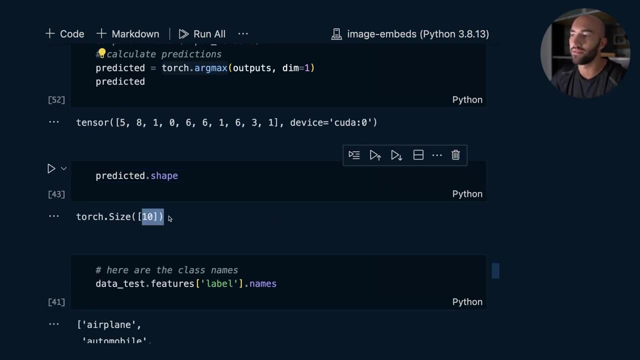 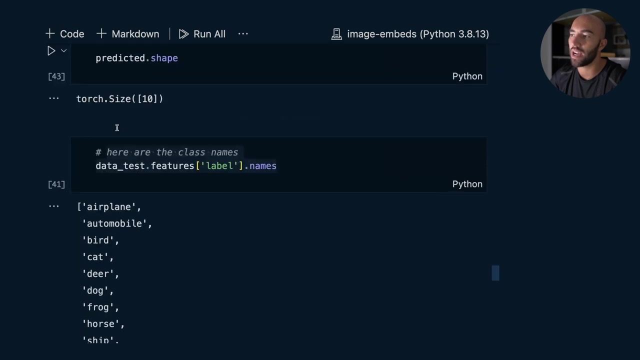 number five had the highest activation. that means the model is predicting that this model is. whatever class number five is. we'll see what that is in a moment. we can just see the number of predictions we have here. it's 10.. so we can see the class names. so here, if we look at this, the number five would be zero. one, two, three. 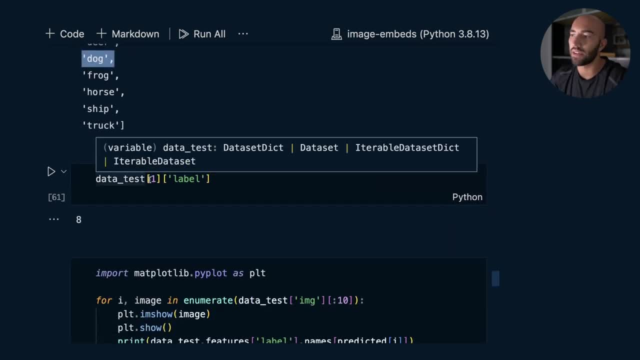 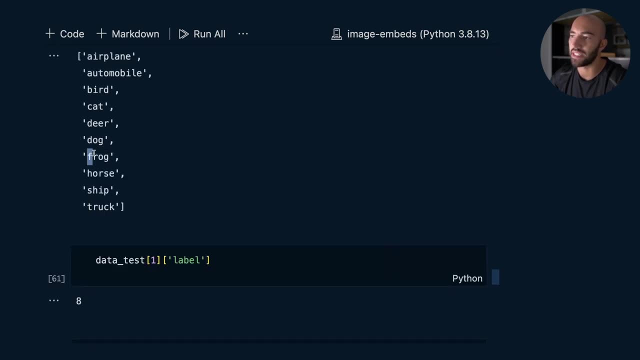 four, five. so the first one is predicting dog and, if we have a look here, the second one is number eight. so number eight here. uh, we'll go a little further. so six, seven, eight, ship. we come down here and what we can do is find the predictions for. 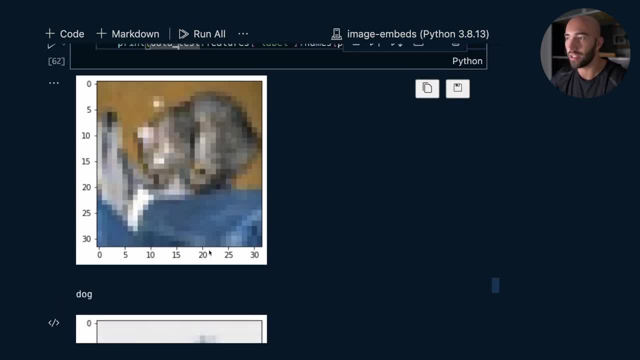 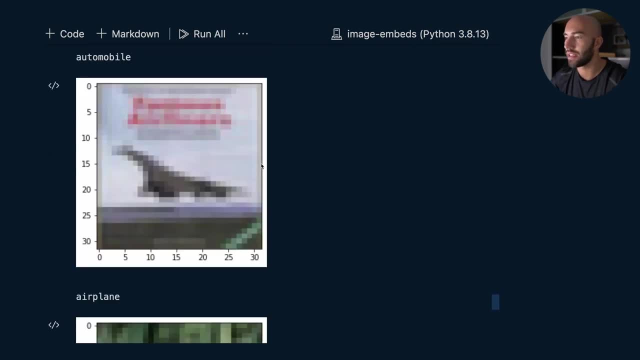 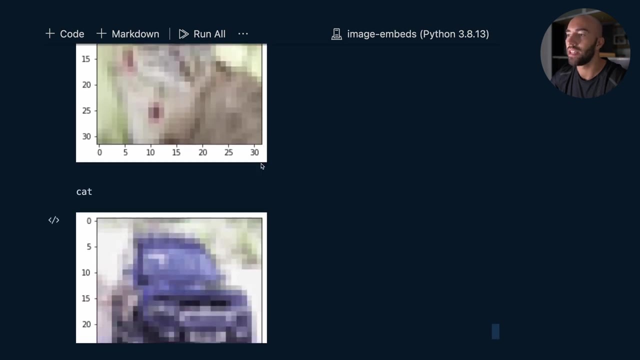 one of these. so this one is apparently a dog. it's pretty hard to tell, to be honest. this one is a ship, a automobile- which maybe isn't accurate- an airplane, a frog, another frog automobile, and so on and so on. so, generally speaking, most of those actually do look correct. so we have 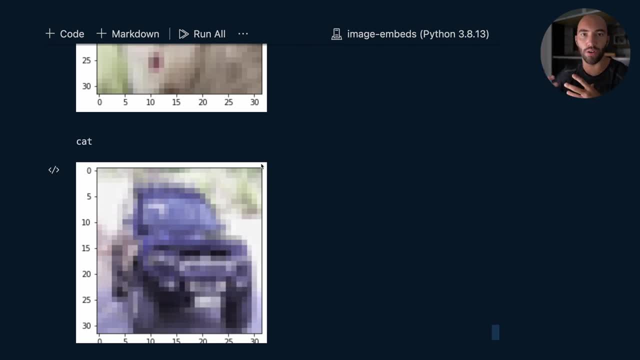 successfully managed to train our convolutional neural network on this classification task for images, and that is despite these images being very low resolution. like even myself as a person, I struggle to figure out what exactly is in each one of those images. but that's it for this. 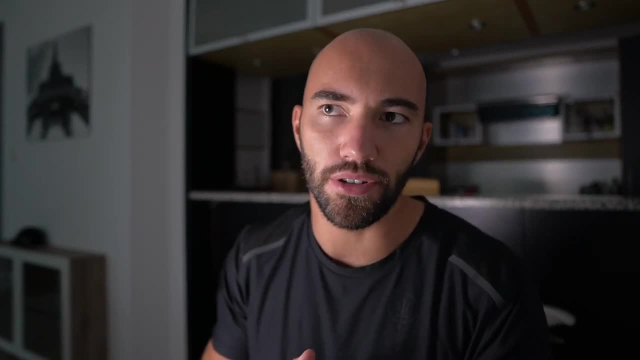 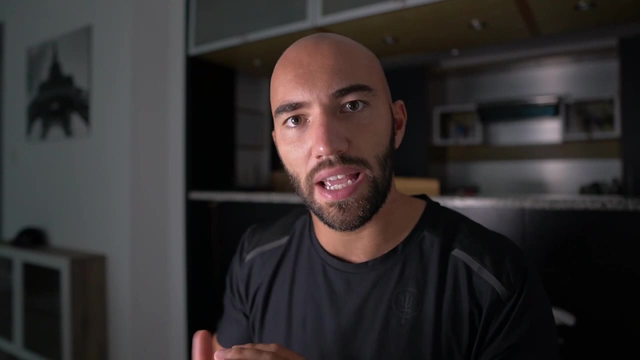 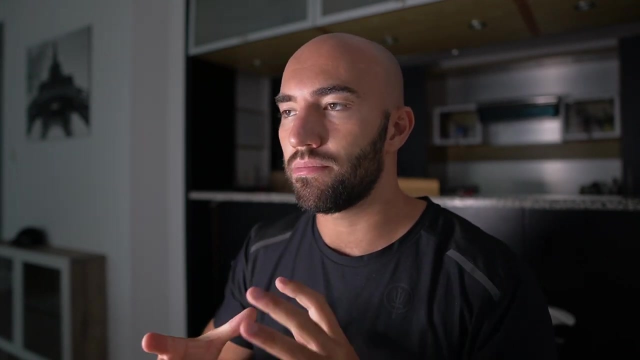 introduction to the long reigning champions of computer vision, ie the convolutional neural networks. we've gone through the intuition behind these models and had a look at a few of the most popular versions of these as well, which should always inform us as to, you know, if we wanted to build a convolutional neural network. 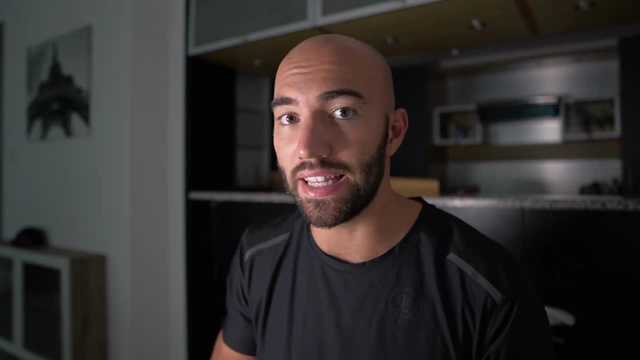 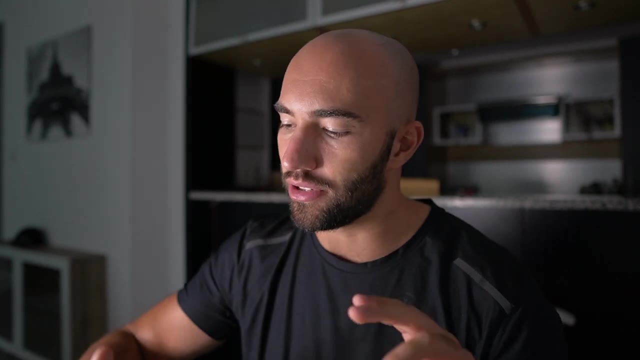 always have a look at those past implementations of what they did, or just use one of those out of the box. and then after that, we obviously went through all this code went through actually, uh, training a convolutional network and actually using it for inference as well. so, as I said,